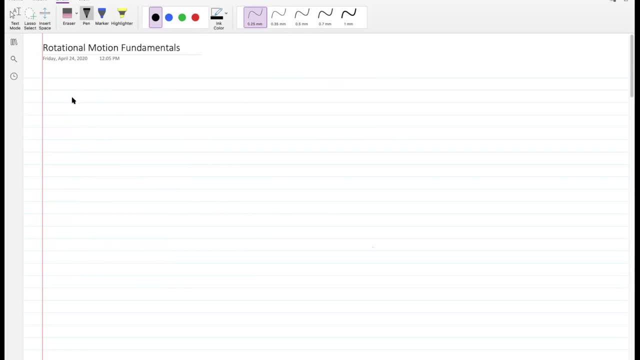 Hi there, I'm going to cover some rotational motion fundamentals for students that are taking the Physics C exam. So let's get started. I have copied over the relevant equations from your equation sheet here. And one thing I would like to re-mention, as I did in my last. 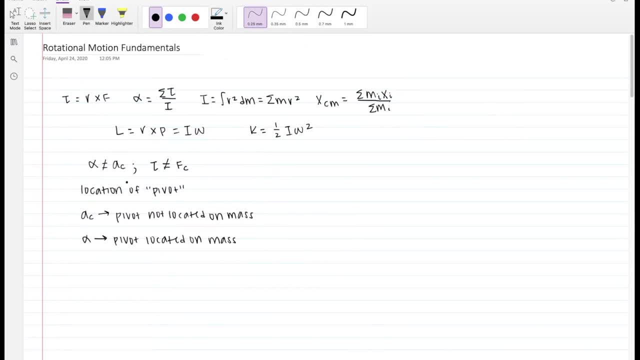 video about circular motion is that angular acceleration is not equal to centripetal acceleration and torque does not equal to centripetal force. It depends on the location of your pivot. So for centripetal acceleration, your pivot is not located on your mass. 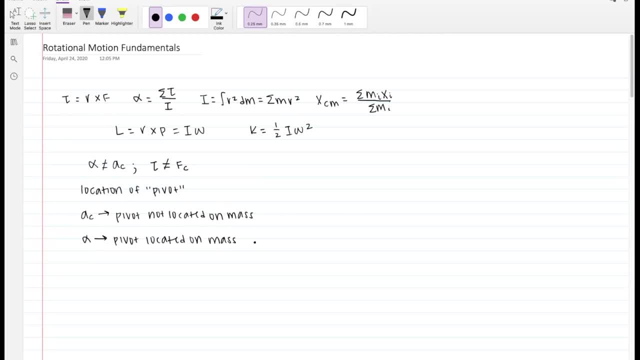 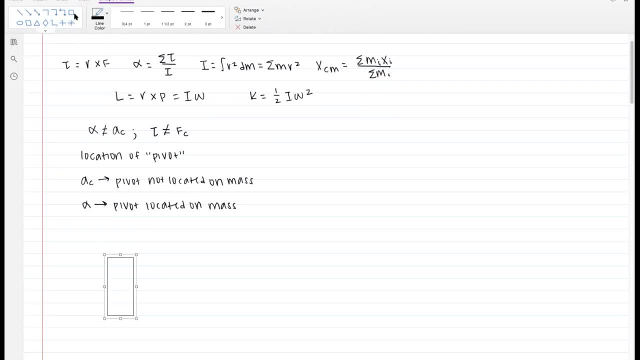 and as for angular acceleration, the pivot is located on your mass. Let's say that we had a block and the center of mass is located here. Torque is equal to the radius times, or cross product, really, of your force. Your radius is the distance. 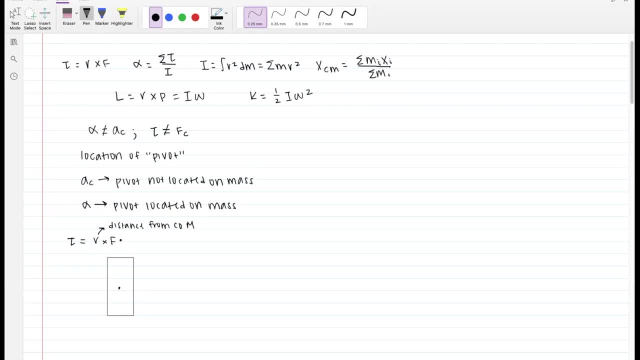 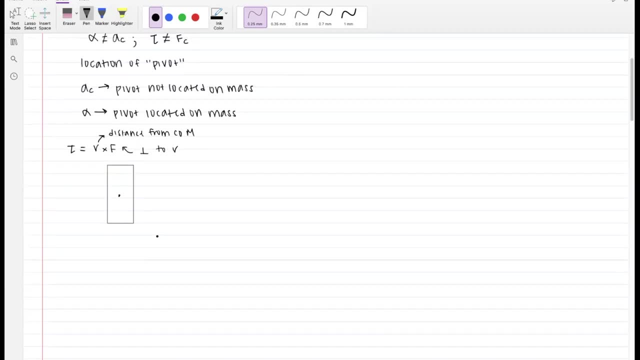 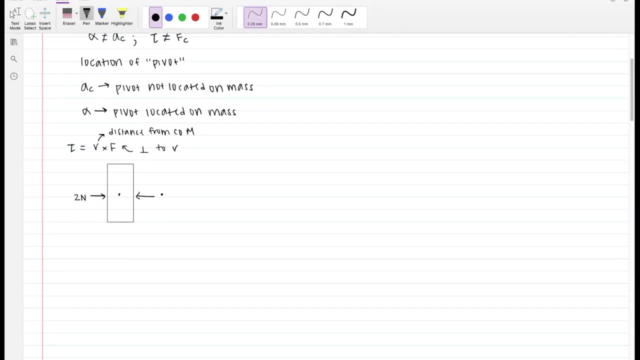 from your center of mass and your force is going to be perpendicular to your radius. So let's look at this example. Let's say we apply two newtons at the center of mass and let's say we applied another two newtons on the opposite side, at its center of mass. 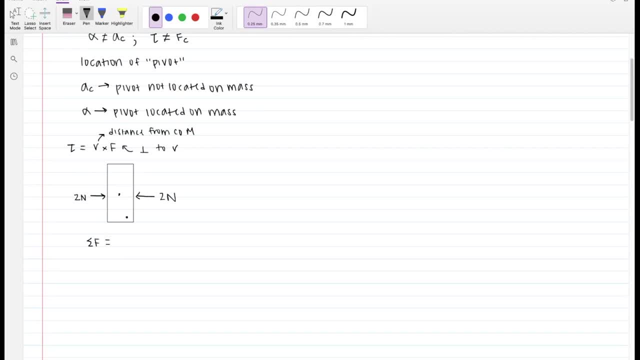 The sum of all the forces is equal to two newtons to the right- we're going to consider that positive- and two newtons to the left, which we're going to consider negative. Well, that gives you a net force of zero. And let's look at the torque. 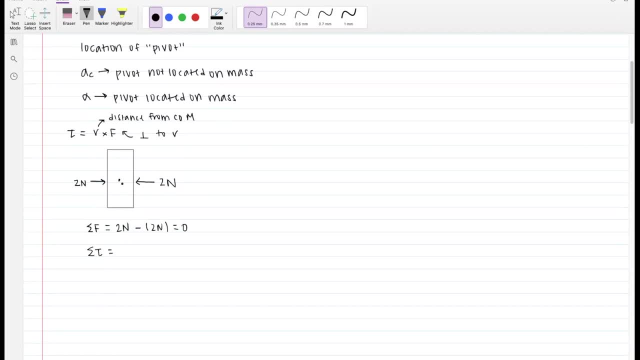 The torque is equal to well, the distance from the center of mass is zero because we're applying the forces at the center of mass. so two times zero and same for this case, and we're going to keep this connotation negative, since the forces going to the left 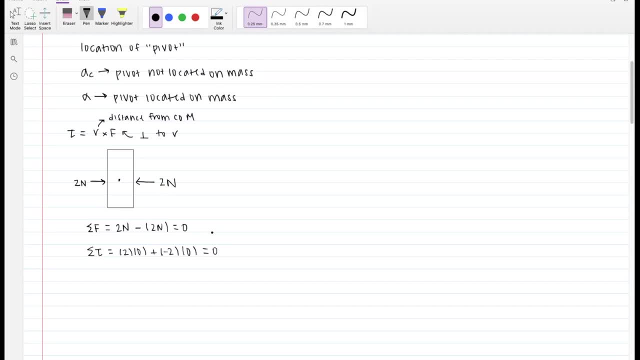 Zero. All right, so you could. All right, so this block, and if you try this at home with a pencil, the sum of the forces is going to equal to zero and your pencil is not going to rotate. Now let's look at it this way: 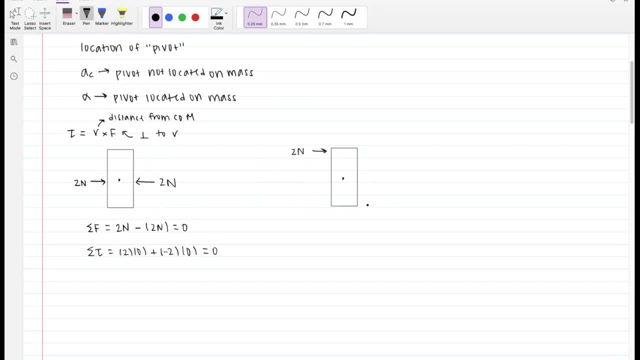 We have two newtons going to the right and two newtons going to the left, and let's say that the entire height of this block is two meters. so that means it's going to be one meter going up and one meter going down. 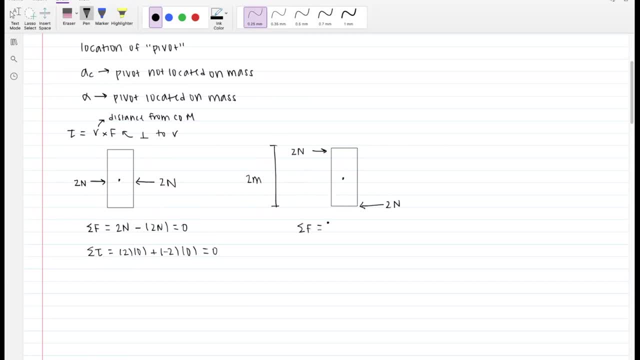 Sum of all the forces. Well, we have two newtons going to the right, two newtons going to the left. Well, that's going to equal to zero. Let's look at our torque: We have two newtons going to the right and we have the radius. 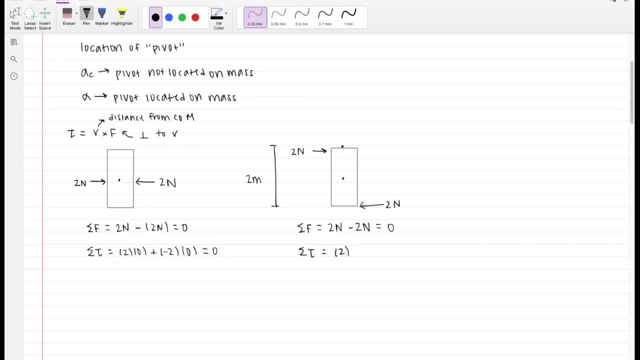 so the force that's being applied is perpendicular- perpendicular to its radius, so that's one meter. and then we have two newtons applied here to the left, so that's negative and because we are working in the opposite direction, it's going to be negative one meters. 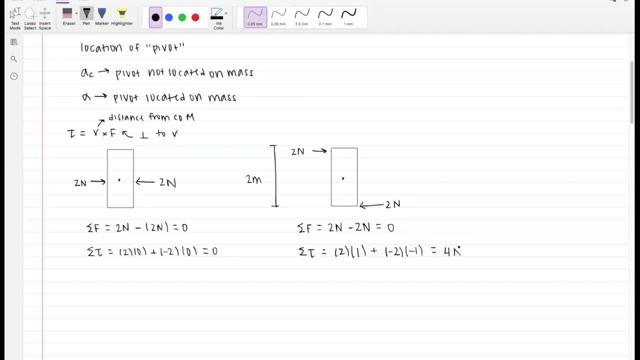 So that's going to give you a total of four newton meters, And if you try this at home, you'll see that this block will rotate clockwise And from now on we're going to consider clockwise motion as negative and counterclockwise. 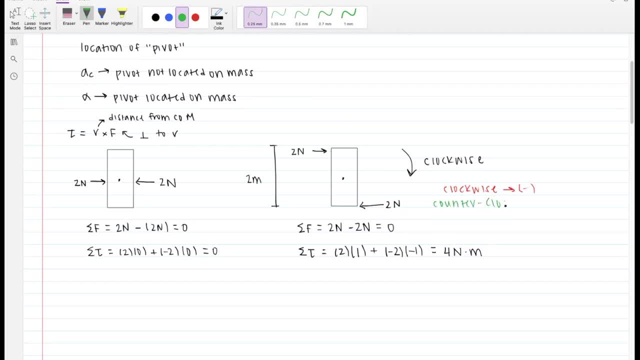 as positive, So technically this should be negative. four: Again: if directions are confusing for you, you don't need to keep to this convention. One can be positive and the other can be negative, or you can just consider both of them as positive magnitudes. 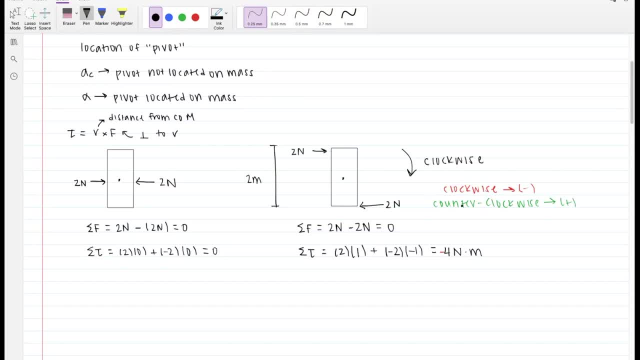 However, whenever you do work with torque, you have to understand that these are opposing motions. We'll talk about that in the example I have here. Let's say that you have this example here, where we have a beam and a fulcrum. 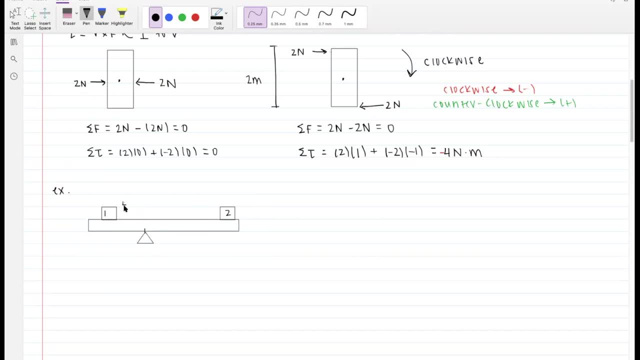 and we have block one and block two. let's say that we know the mass of block one, let's say four kilograms. Let's say that this block is positioned 0.2 meters to the left of the fulcrum and this block is positioned 0.6 meters from the fulcrum. 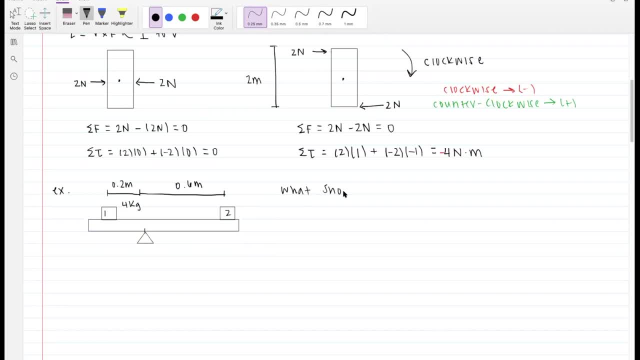 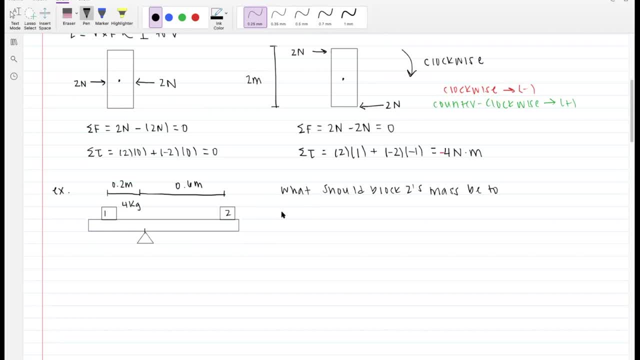 processes where there is greater mass cannot 주면. process where there is greater mass cannot 주면, keep equilibrium And that's the key word: equilibrium. We have equilibrium of this system. that means that all the forces, and most especially the net torque, and most especially the net torque, 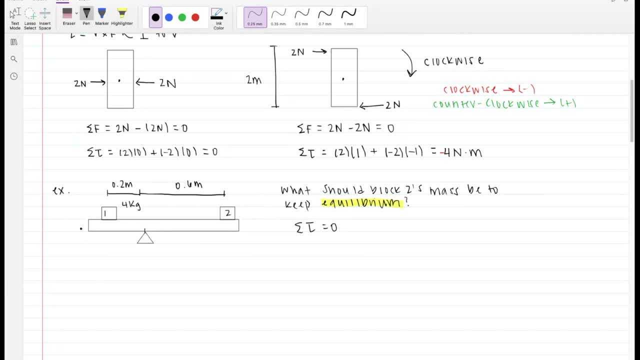 is equal to zero. Let's draw an FBD for this. So we have the force of gravity applied on block one, the force of gravity applied on block two. Now the beam itself also has a force of gravity being applied to it. however, we're going to 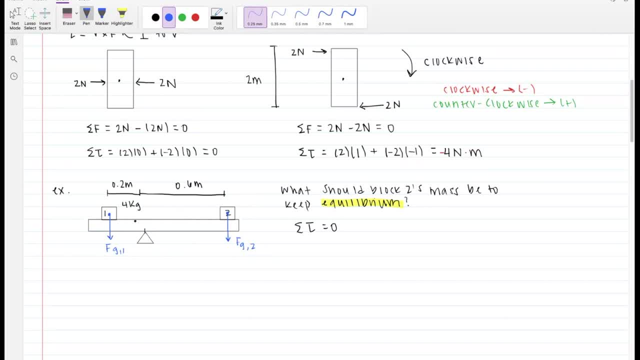 talk about that in the second step of the problem. Let's make also this fulcrum the zero point. Well, if you look at this, this block one, this is going to provide a torque in the counterclockwise direction and this force is going to provide a torque in the clockwise direction. 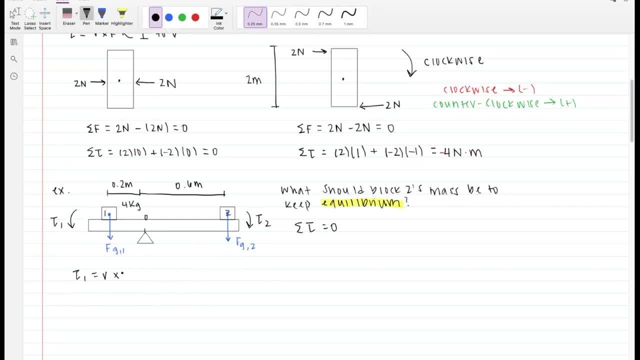 Now let's calculate torque one, which is our cross product F, So our radius is zero point two, And our force is mg, so that's going to be four kilograms times ten or nine point eight. but let's round for this case. 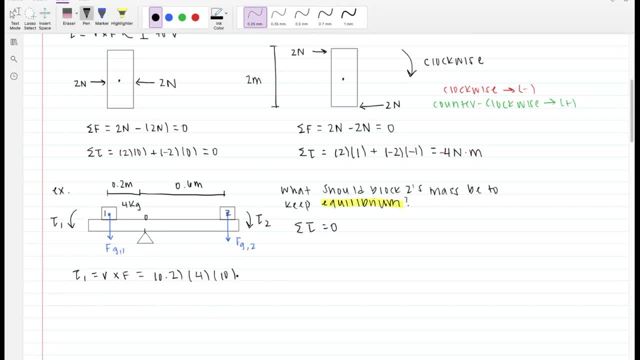 As you can see, I didn't apply direction to these vectors. however, we're going to keep to this connotation that clockwise is negative and counterclockwise is positive. So after this calculation, we get eight newton meters And because this is producing a counterclockwise motion, we're going to assign this as positive. 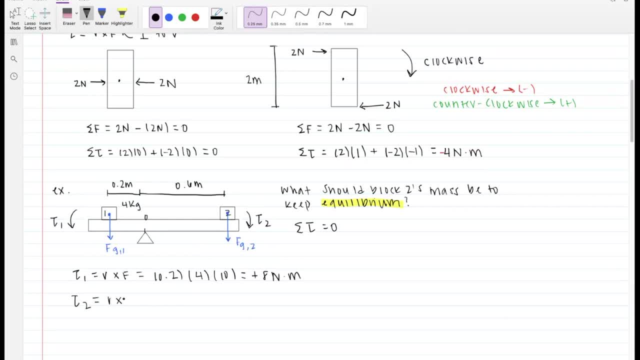 Now let's calculate torque two. we have a radius of zero point six. we have some sort of mass that we don't know and gravity. This is going to give us six times some sort of mass, m. this is going to be newton meters. 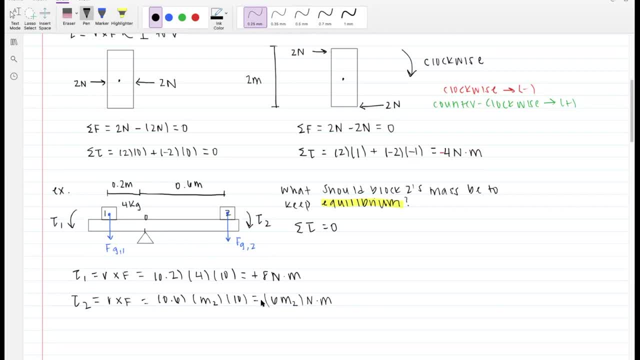 And because this is producing a clockwise motion, we're going to assign that as negative. So summation of all the torques is equal to torque one plus torque two, which is equal to eight minus six m two, which is supposed to equal to zero. 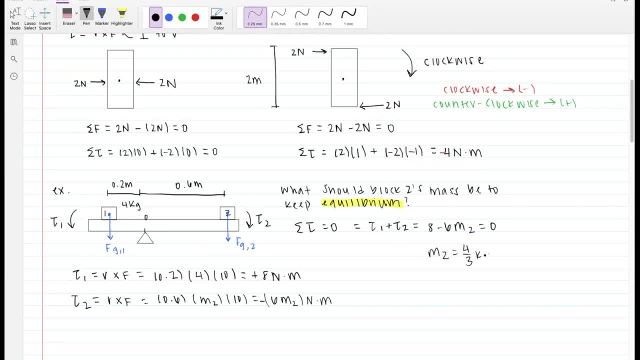 That means that mass two has to equal four thirds kilogram. Again, if this connotation is really difficult for you to understand, maybe think of it this way: The torque and the counterclockwise the magnitude needs to equal the torque and the. 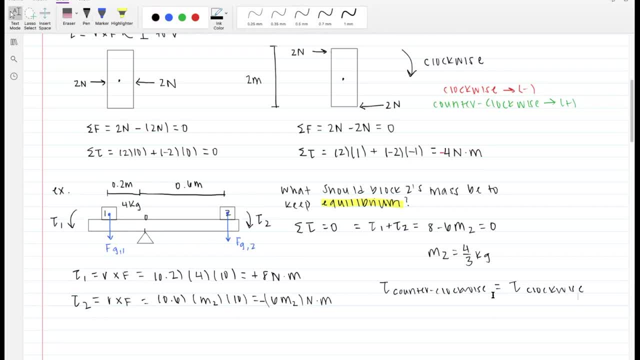 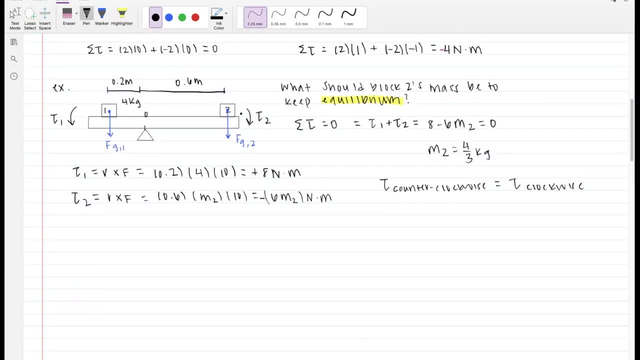 clockwise motion. What this will do is it will allow you to not have to assign negative or positives. Okay, what if you were given the question: what is the system's center of mass? Okay, Okay, Okay, Okay, Okay, Okay. 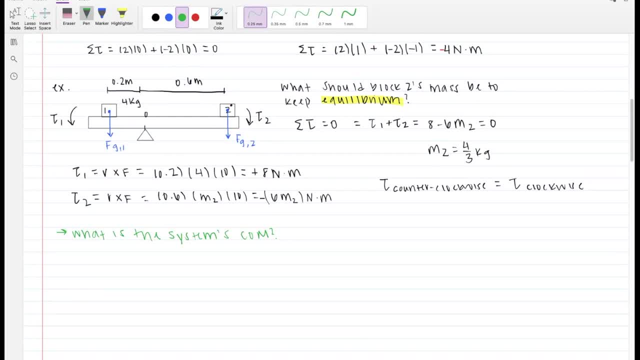 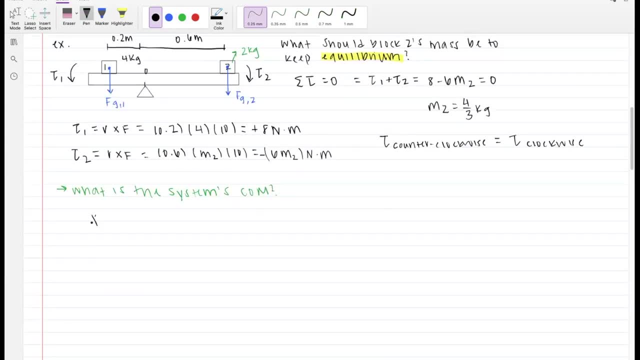 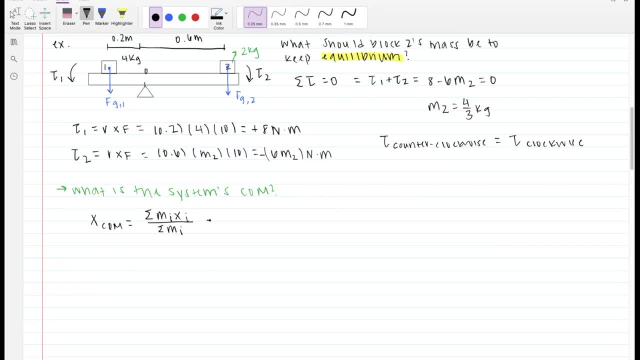 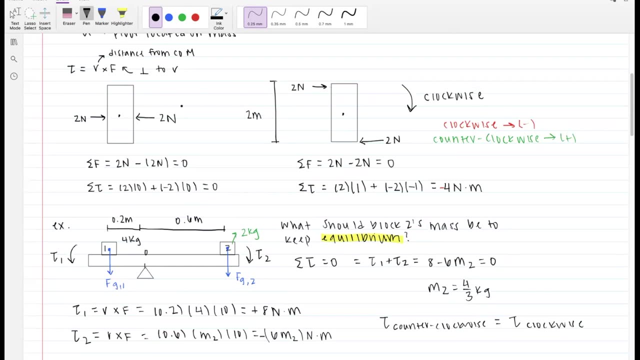 over the sum of the masses. Now, for this you do need to assign direction and you do not care for torque, but you do need to care about the torque direction of your forces, as i did in this scenario. so the mass of the block is four kilograms. 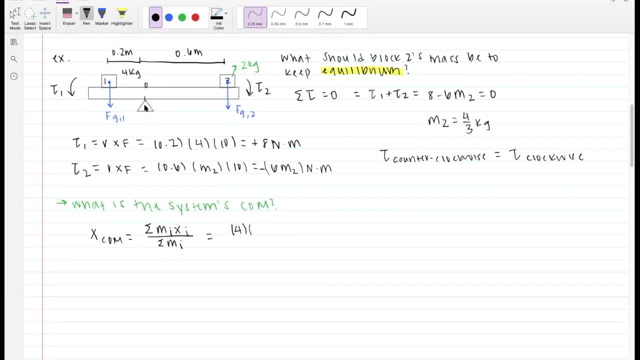 and we have the distance from the center point, which is zero, at the fulcrum and to the left, so that's going to be negative 0.2 meters. plus we have mass 2, which is 2 kilograms, and it's 0.6 to the right, so it's going to be positive 0.6. 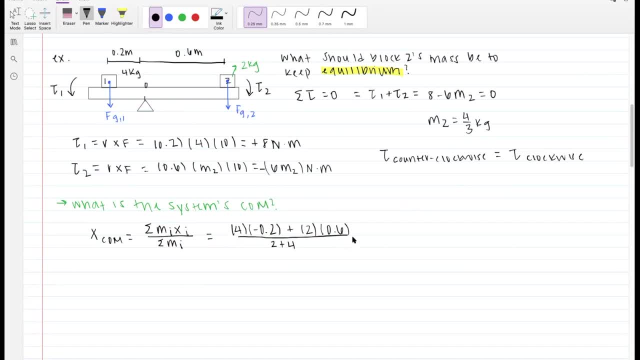 all over the total mass, which is 2 plus 4.. this is going to give you plus 0.4 over 6, which is equal to 0.067 meters. so that means 0.067 meters to the right of the fulcrum, and what that does is then causes the torque to not equal to zero. 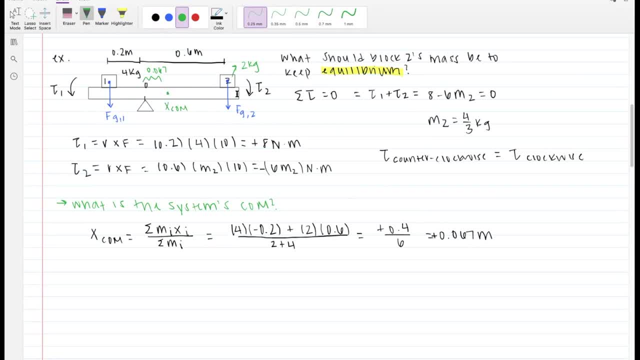 and what will happen is that you'll see a rotation and this block will then go down, while this block will go up. whenever you see a problem like this, the center of mass is at the fulcrum, when in equilibrium. now, if you redid this problem where you assigned instead four thirds for the mass instead of 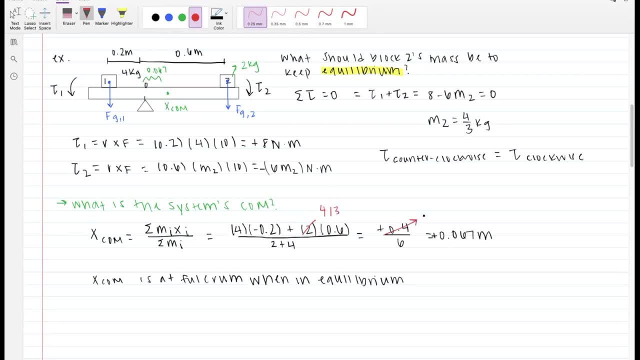 two, you will get zero, and therefore the center of mass is going to be at the fulcrum. that leads me to another point. point gravity, or the force of gravity, is applied at the center of mass. So this beam does have gravity applied to it And in this case the center of mass was at the fulcrum. 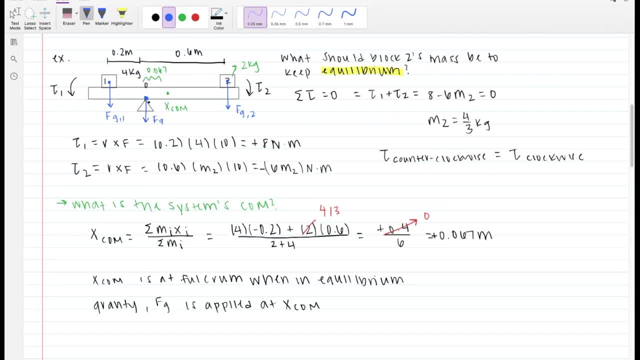 f of g, But this gets canceled out because this is going to be on a surface, by f of n. But if the center of mass is no longer at the fulcrum, the force of gravity will be applied here instead, Hence why block two accelerates down and block one will accelerate up. Let's look at 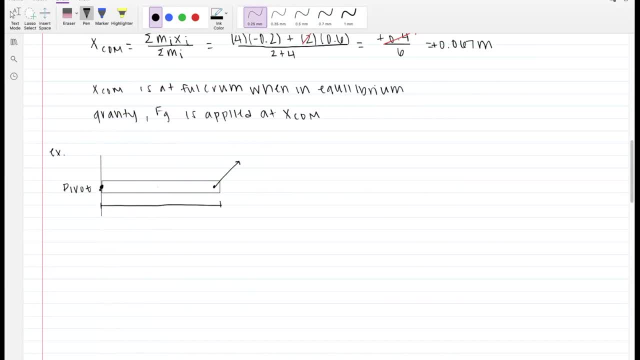 another example problem. Let's say that we have some sort of wall and a beam connected to this wall. We apply a force of 20 newtons at this angle, let's say 30 degrees, And the length of this beam is, let's say, three meters. So what is the net torque acting about this pivot? So let's. 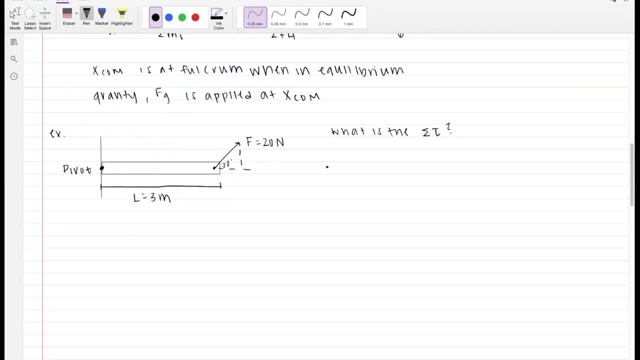 look at this. The first thing you should do is always split up your vectors. So you have f, you have f of x and f of y, And because this is 30, this is going to be f, which is 20 sine 30. 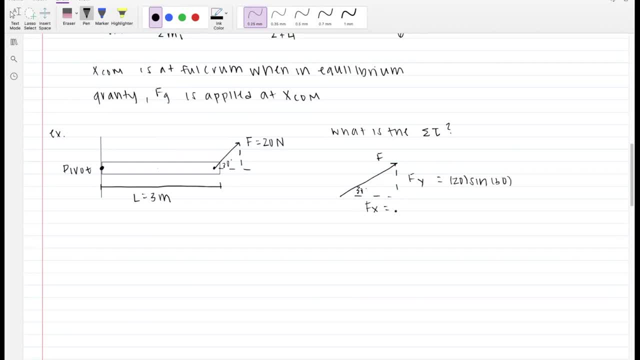 degrees, And this is going to be f. so that's 20 cosine, 30 degrees. And before we do this computation now, I want you to remember the equation for torque or cross product f: The force applied needs to be perpendicular to your radius. This is my radius r, So the only force that is relevant. 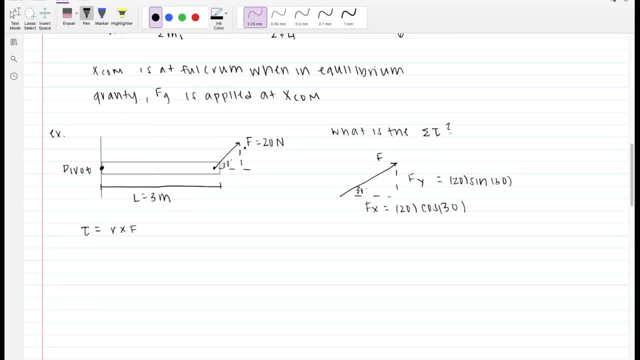 to us by this applied force is the force that's being applied in the y direction. The force applied in the x direction does not matter, Because the direction is not perpendicular to the radius, It's in the same direction. Now, one last thing. There's a force of gravity that is being applied to this beam And, as you can see this, 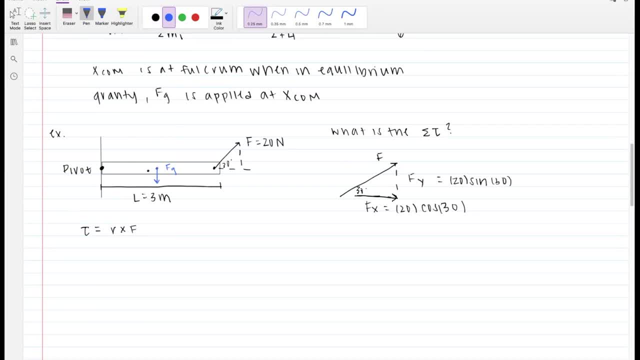 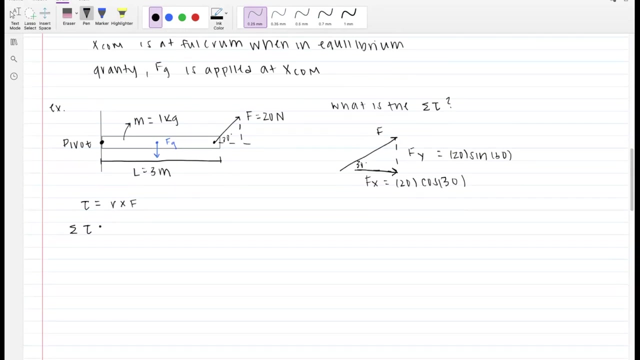 force is being applied in perpendicular to the radius. Now you can consider both f of g and this force applied in the y direction. Let's say that the mass of this beam is equal to one kilogram. Make things simple. So torque, summation of all the torque is equal to r times f. So we have 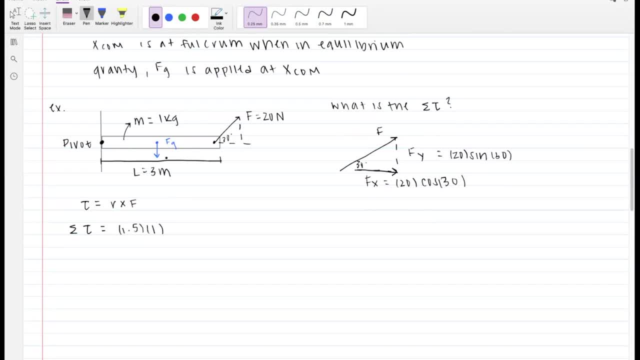 1.5 times 1 times 100 gravity, And this is producing a clockwise motion. So this is going to be negative, plus the f of y times the length here, which is going to be so r of three, force of 20, sine of 30. 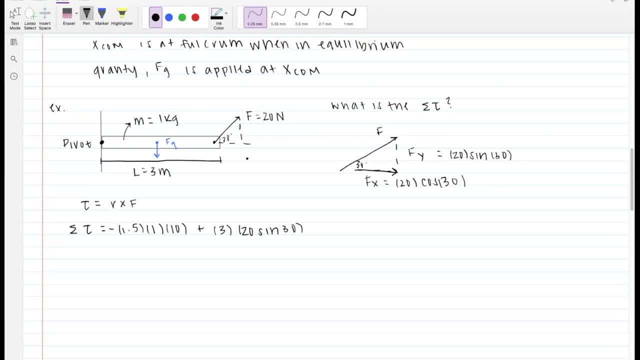 and because this produces a counterclockwise rotation, we're going to consider this as a positive quantity. When we look at this, this is going to give us negative. 15 plus sine 30 is the same thing as one half. So 20 times one half is 10.. Three times 10 is 30.. 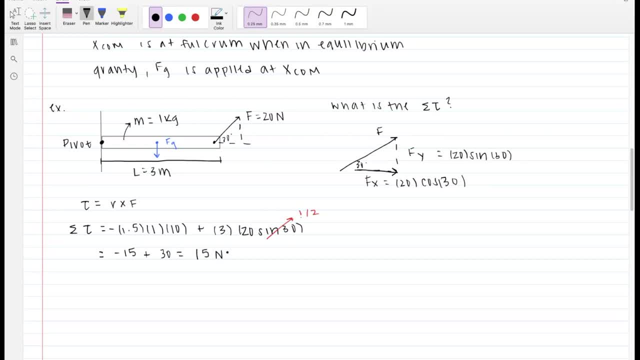 So this gives us negative 15 plus sine 30. So this is going to give us negative 15 plus sine 30. This gives us a net torque of 15 Newton meters. Now let's say, if we're given that I is equal to. 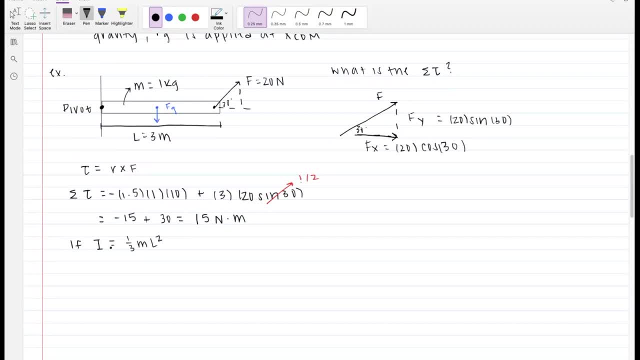 one third and all squared. So this moment of inertia, what is its angular acceleration? Angular acceleration is equal to the net torque all over moment of inertia. That's going to be 15 over one third ml squared, which is equal to 15 over one third, one kilogram and a length of three. 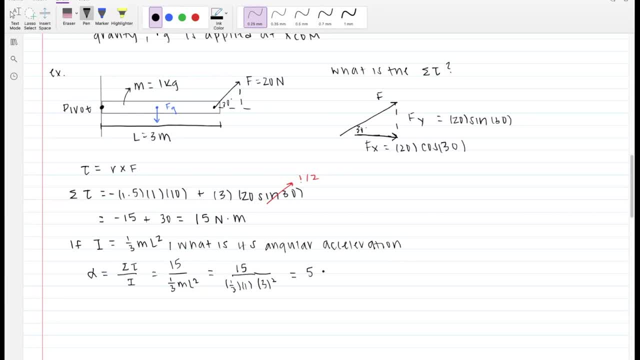 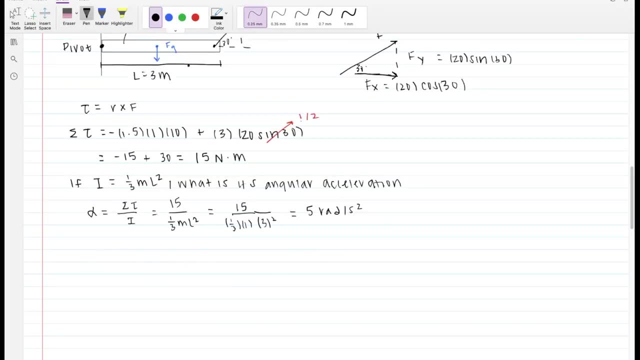 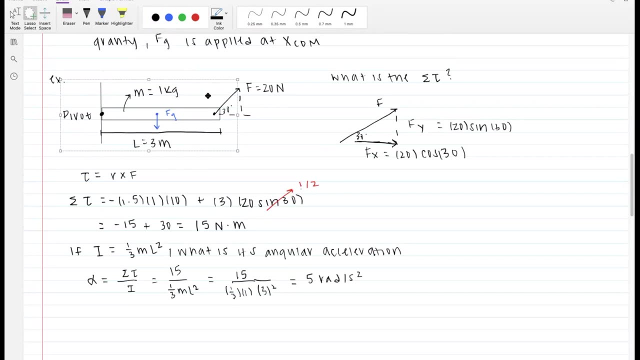 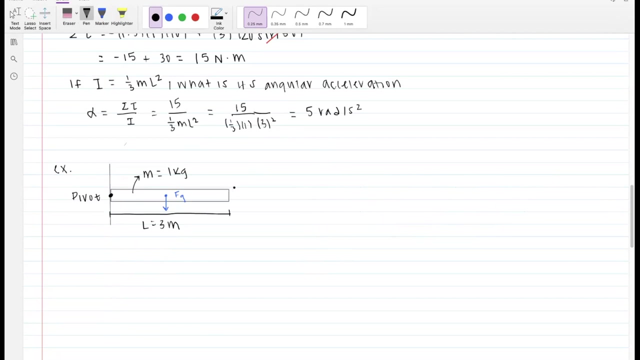 squared, This is going to give us five. So this is going to give us 15. over one third one kilogram. This is going to give us five radians per second squared. Now let's assume that we have the exact same problem, but we don't apply force, And let's say that this rod then rotates. 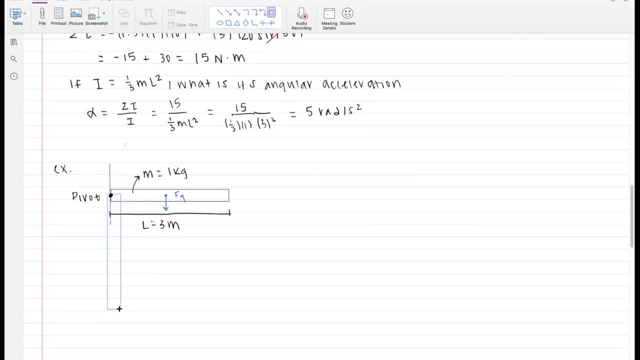 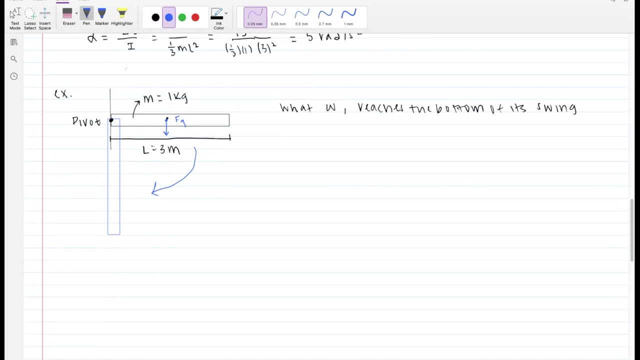 all the way downwards, as so Question that might be asked is: what is the angular speed of which the rod when it reaches the bottom of its angular speed? Okay, One thing I want to make, a huge point, is that we are looking at the force of gravity, which is 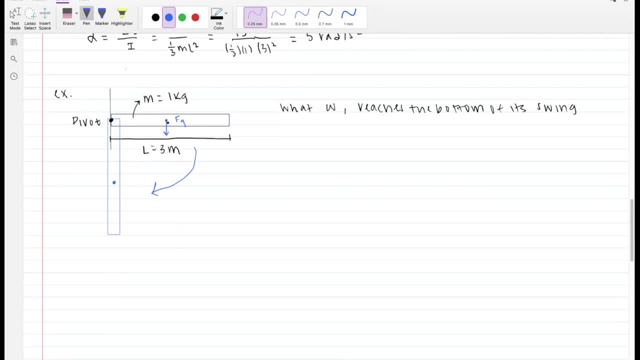 acting on its center of mass, which is halfway in between this rod. So the distance from the pivot point to the force that's being applied by gravity is 1.5 meters, And when we swing at the right position it's going to move along the fossil on the second side. It's not going to move because gravity has a limited power of few meters. but I'm gonna draw this out here, on this surface, right here, where we have thiszeptic, примерно, and that's going to give us a joy of few meters. 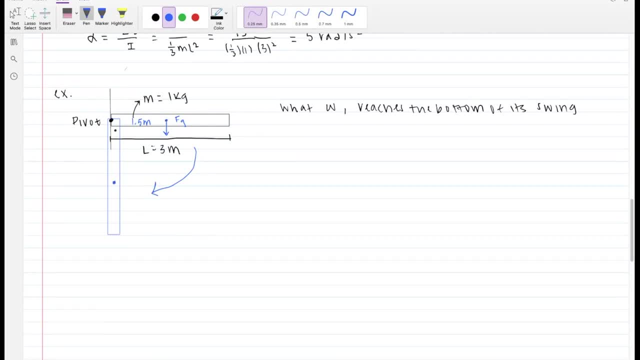 S 요 cynicalnessо this rod to its lowest point. we are going to be looking at the change of distance from its center of mass. The best way to solve this type of problem is a conservation of energy. So we have: change of view is equal to negative kinetic energy or, very simply, the absolute value. 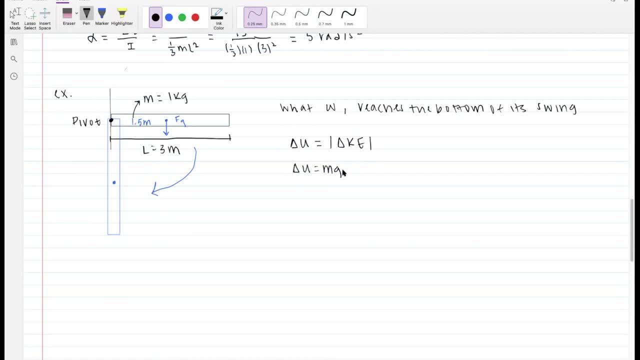 So the change of view is equal to mg, delta H. We have a mass of 1, gravity being applied is 10, and the height that's being changed- if we look at it from the center of mass- is only going to be. 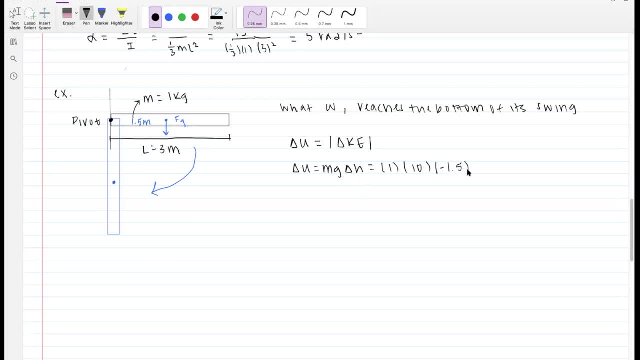 1.5. And because it's going down, I'm going to negate it. So we have negative 45 joules. So our kinetic energy is equal to negative U, which is equal to positive 45 joules. Again, if this really bothers you, having a negative sign for potential. 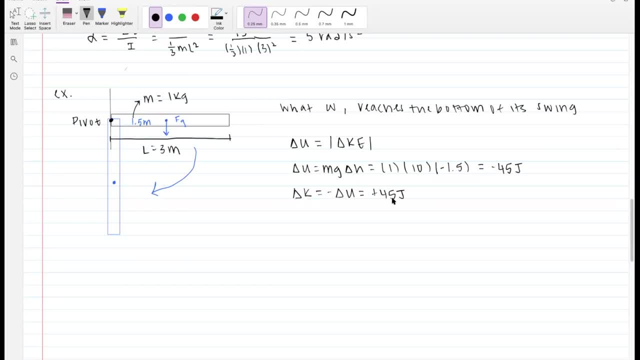 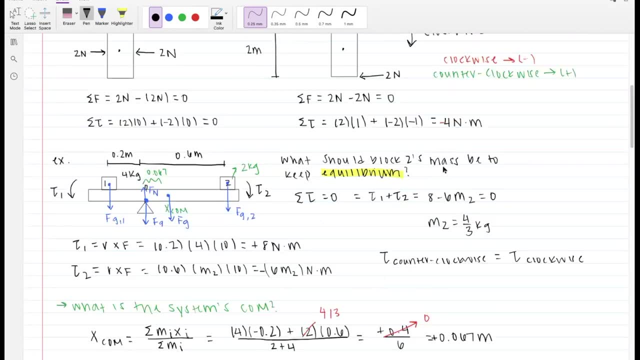 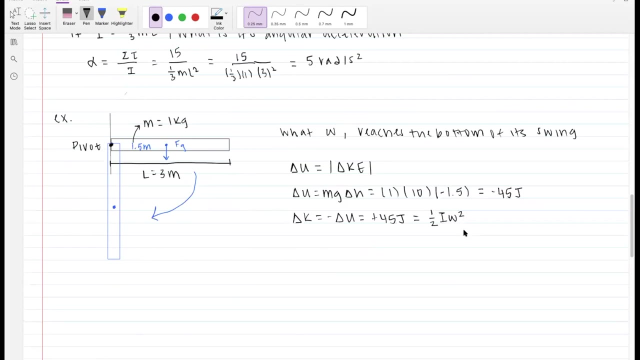 energy. that's fine. Just remember that kinetic energy has to be positive. So we have: this is equal to 1 half. we look at our equation sheet: 1 half moment of inertia, W squared. So our angular speed is equal to root 2 Delta K all over. 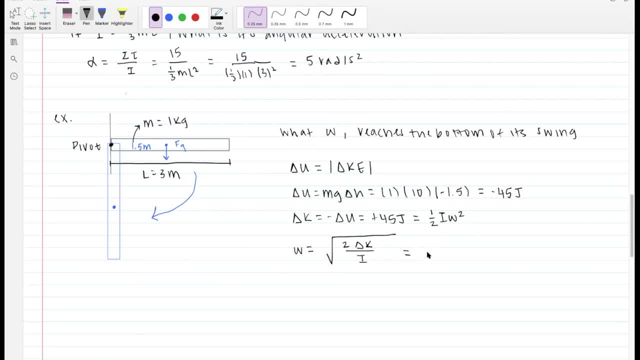 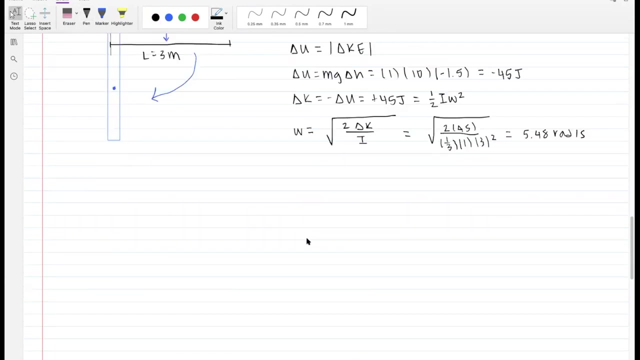 moment of inertia. This is going to equal to root 2 times 45 joules, all over one third mass times length squared. So this is going to give us 5.48 radians per second. all right, so this is going to segue into talking. 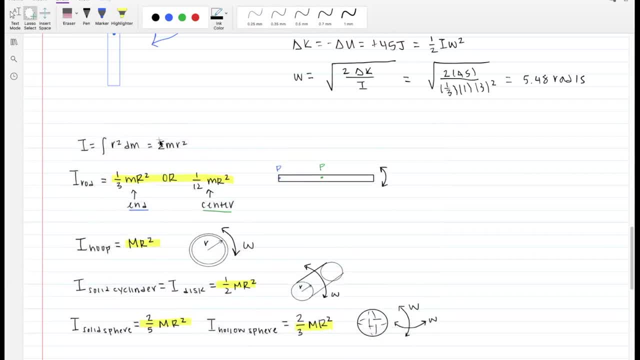 about moment of inertia. so we have this equation: that moment of inertia is equal to the integral of R squared DM, which is equal to the summation of M R squared. now there are some very common moment of inertia problems that they use for the physics exam. if you have troubles with deriving these, I would 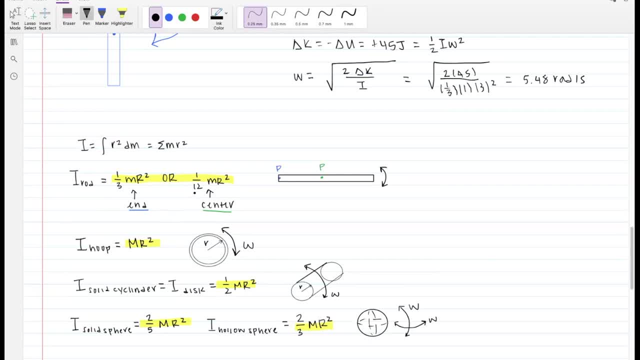 highly recommend that you have these memorized and if you don't have problems with driving them, I would have them memorized anyways because, if asked on the multiple-choice, you don't want to spend time doing derivations for the moment of inertia for a rod when you can just have it. 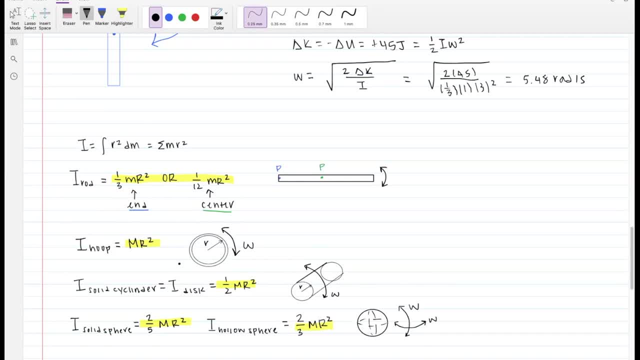 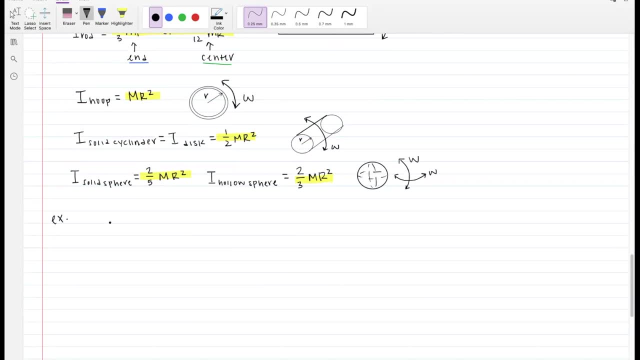 memorized. I'm not going to talk about how I derived these expressions until the next video. a very common example that you might see for both multiple choice and free response, or a small portion of the free response, is if let's say that you were given a rod and we do have the pivot point located at the end. so very 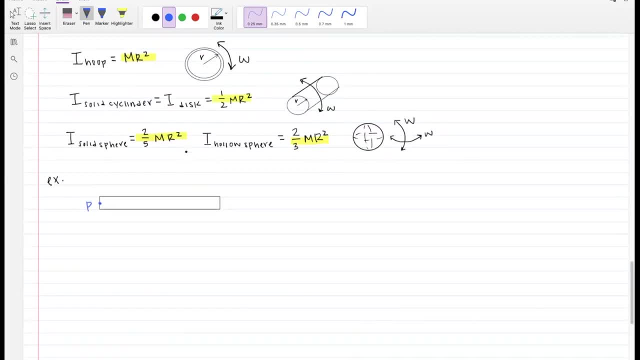 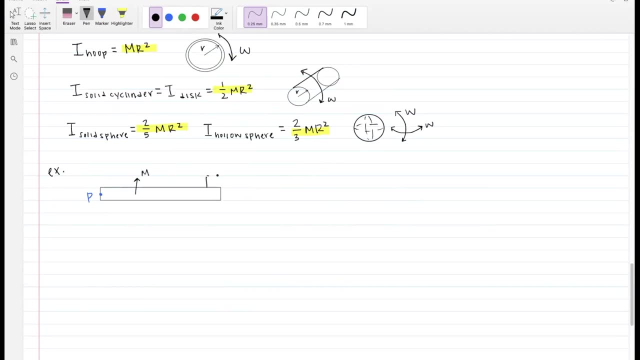 similar to the moment of inertia. So we're not going to be able to do any of these expressions here. We're going to be able to do something similar to the problem that we have here. Let's say that you have this beam with a mass M, and let's say that you have 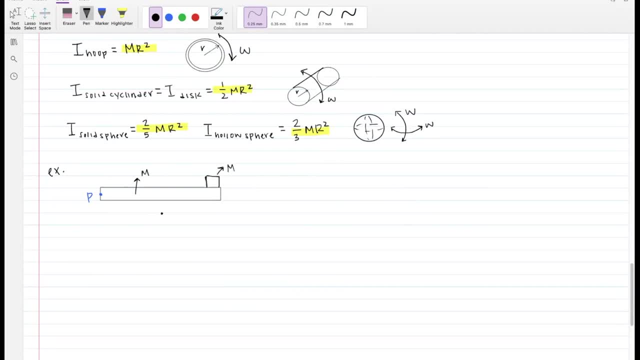 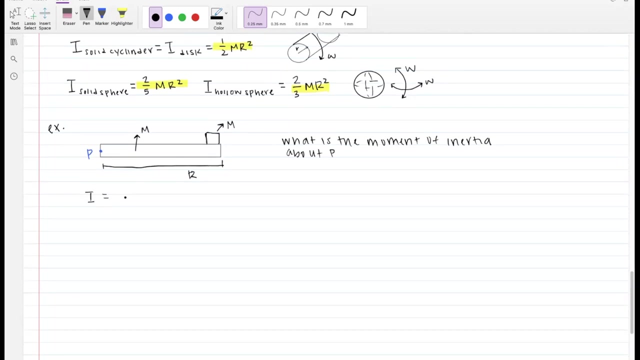 another mass located at its end with also the same mass, and this is with some length of R. and if you were asked what is the moment of inertia? inertia about the pivot point P. So your moment of inertia is going to be the sum of M R squared, So that's going to be the rod, the moment of inertia of your rod. 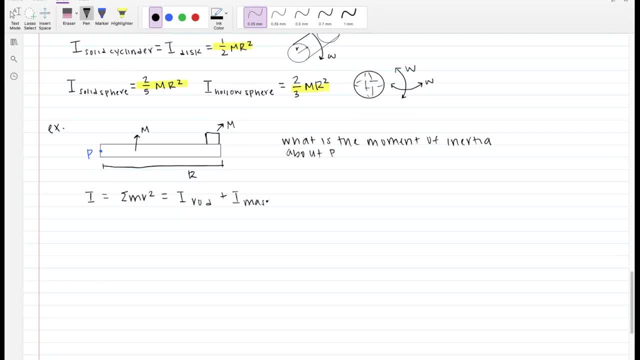 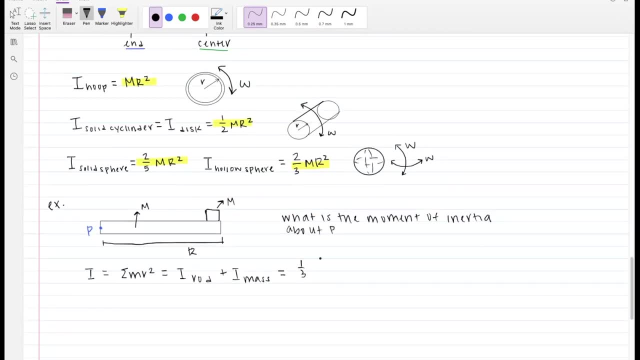 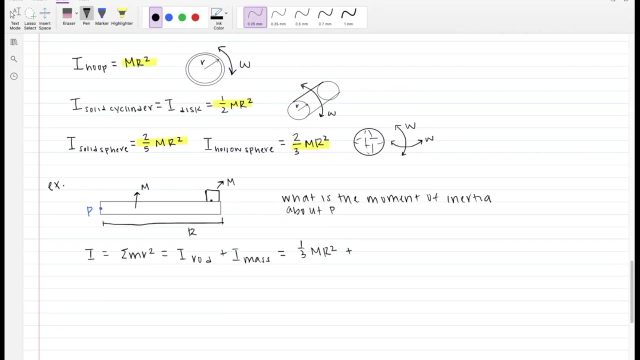 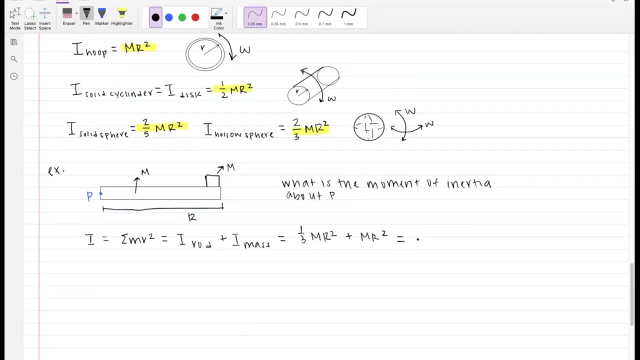 plus the moment inertia of your mass that's located at its end. Well, we already have this memorized, so conveniently. So this is equal to one third M R squared. And then this mass, because it's located at a distance R it has a mass of M, is equal to M R squared. So this is going to give you four. 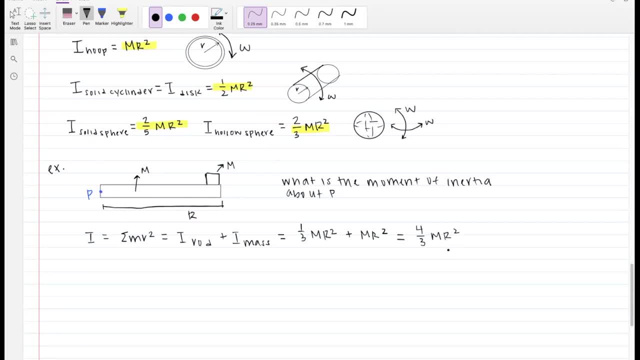 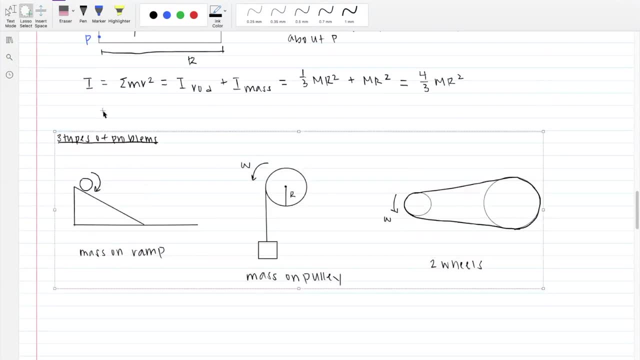 thirds, M, R squared. Now let's talk about some other common types of problems that you will see, Either that they'll be on the free response type, they'll be on the free response, or they could be just a multiple choice question. However, mass on. 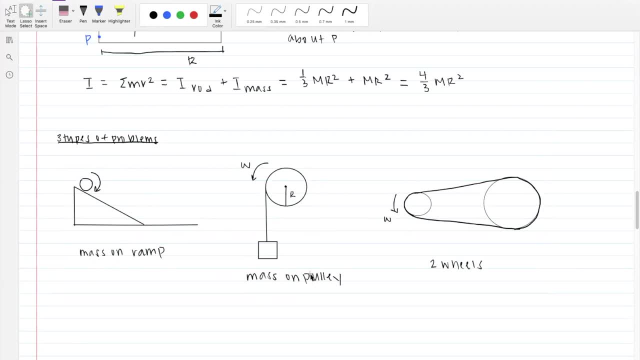 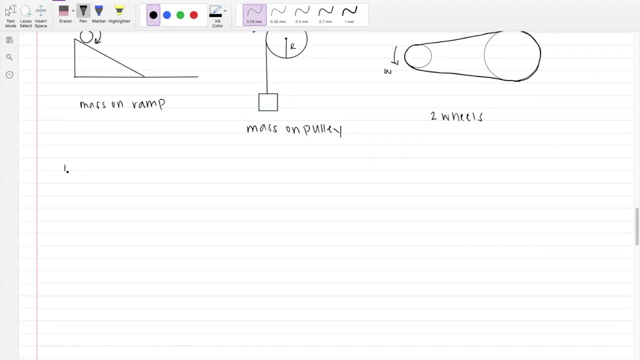 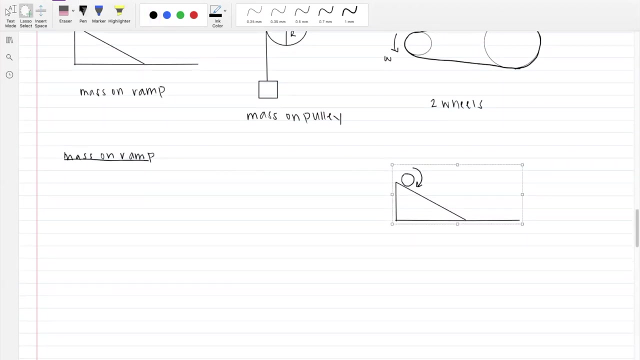 a ramp and mass on a pulley are very, very common to see on free response. So let's look at the example for mass on a ramp. Let's say that this is a 2 kilogram ball. This is a height of 20 meters And it is 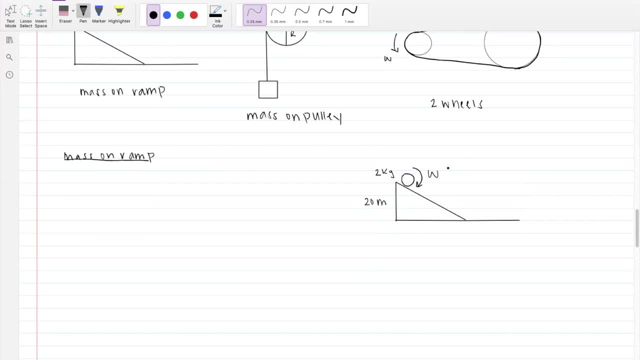 rotating without slipping along this surface. When you look at kinetic energy, you should always consider that kinetic energy is equal to one-half M v squared plus one half IMX squared. Okay, Now the reason why we have not considered this portion in previous problems in kinematics. 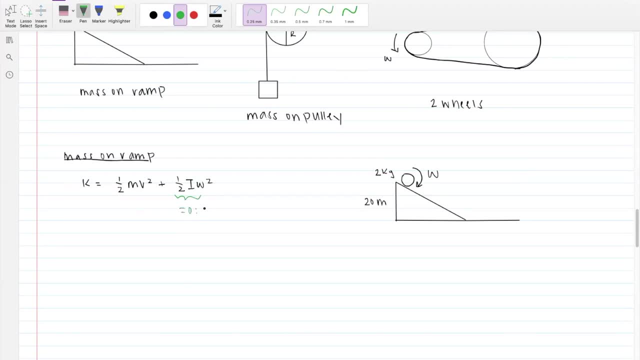 is because this was usually set to zero, because the change in angular position was zero, And for this we should consider this to be equal to zero. only if the change in distance is equal to zero, However, we can see that this ball is changing in distance as well as changing in angular. 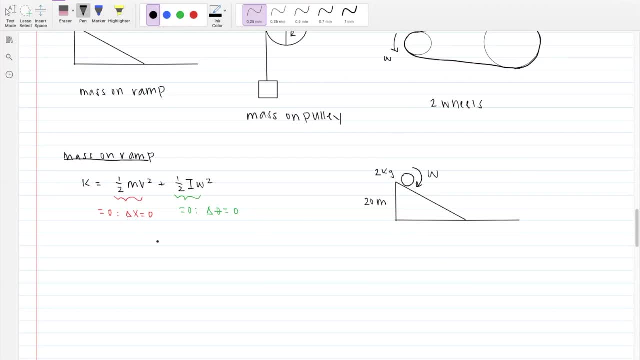 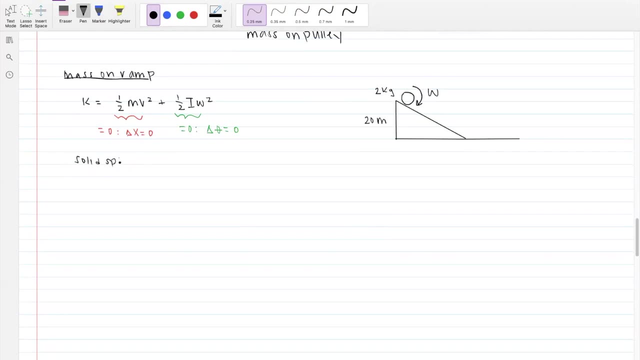 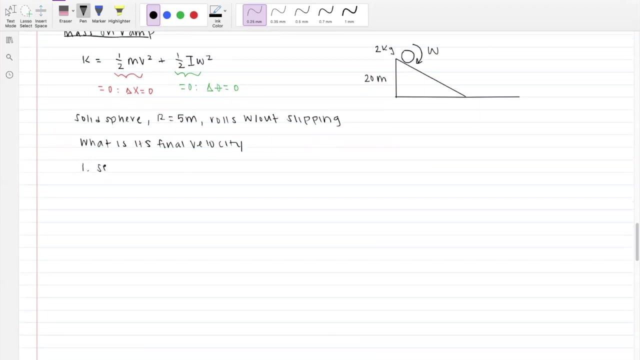 position. So we need to consider both for this problem. Let's say, if we had a solid sphere And it has a radius of five meters and it rolls down the hill without slipping, What is its final velocity? The first thing you want to do is solve, for delta u is equal to negative delta k. 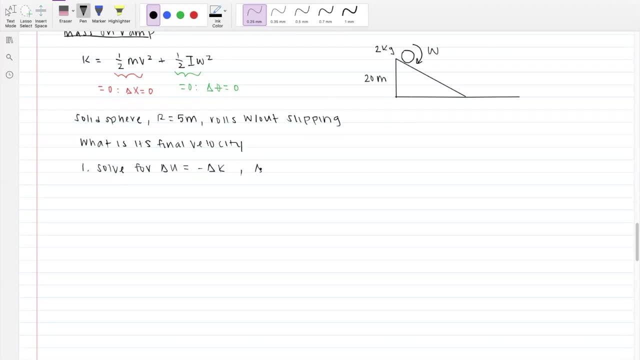 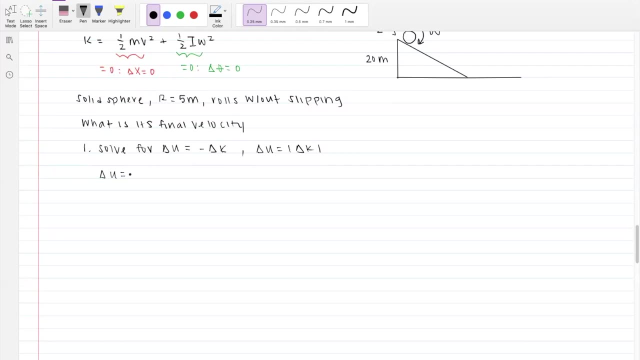 Again, if this is too difficult for you having the signs, just remember: delta u is the absolute value of delta k, So delta u is equal to mg, delta h, which is equal to two times 10.. And we are going to solve for delta u. 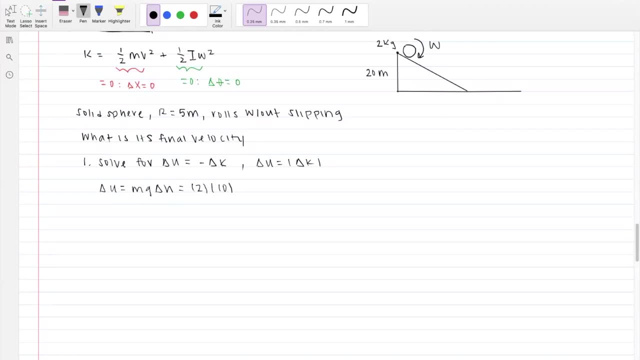 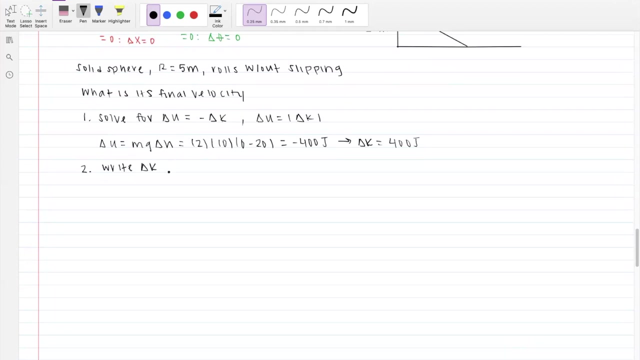 We are going from an initial position of 20 meters to a final position of zero, so zero minus 20.. That gives us negative 400 joules, So our kinetic energy is equal to positive 400 joules. Next you want to write a change in kinetic energy and substitute: 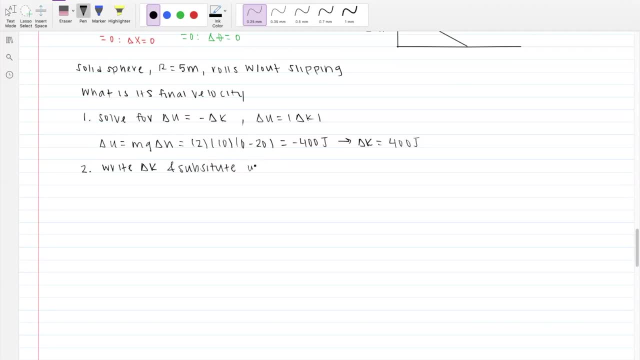 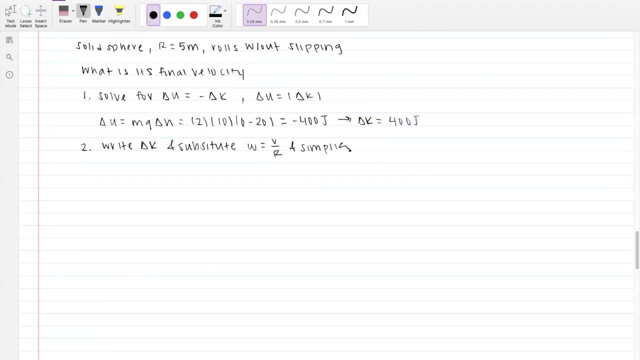 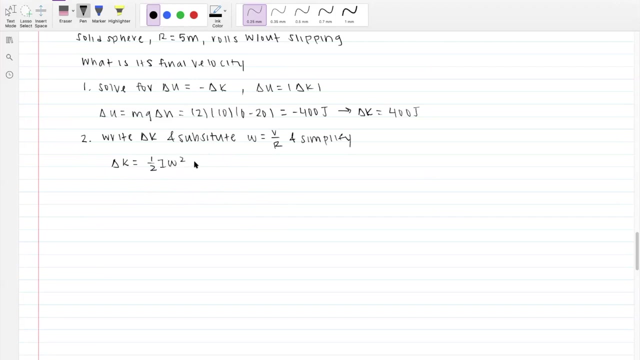 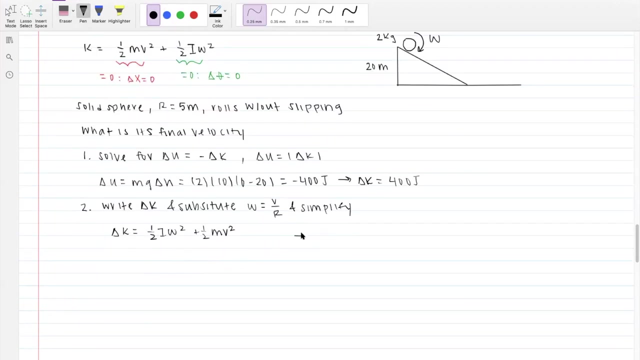 W is equal to v over r, And then we are going to simplify. This is going to equal to one half of the inertia w squared plus one half m v squared, And our moment of inertia for a solid sphere as we look back at our table is equal to: 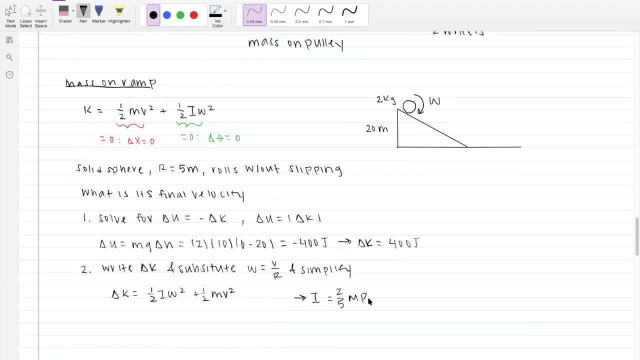 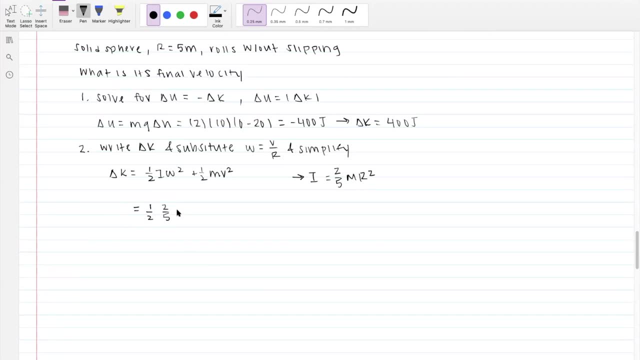 two fifths m r squared. I'm going to go ahead and substitute these variables. So one half times two fifths m r squared W squared will now be v squared over r, plus one half m v squared. Well, very simply, you can see that the r squares are going to cancel out. 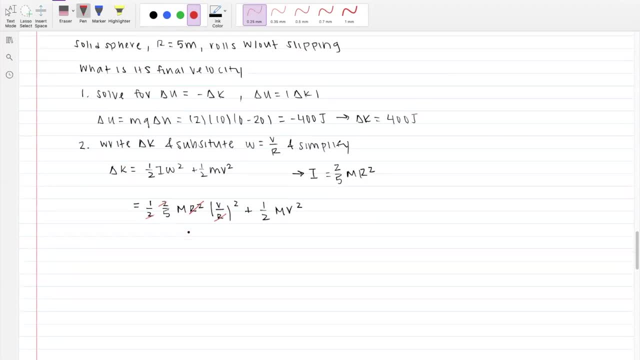 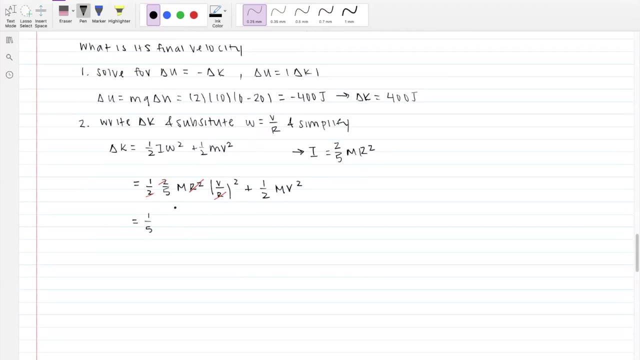 These twos are going to cancel out. Let's plug in the rest of the variables. So now we have 1 fifth mass of 2 kilograms V squared plus 1 half m, which is 2 kilograms V squared, is equal to delta K. 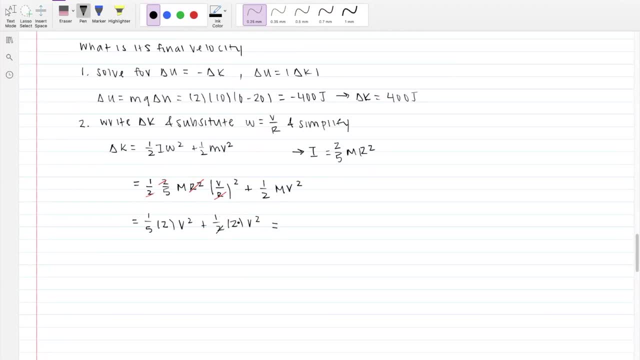 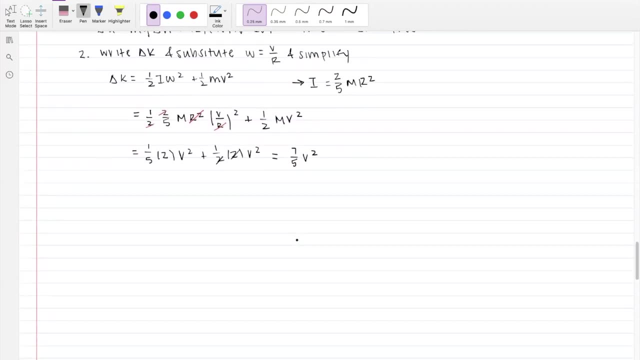 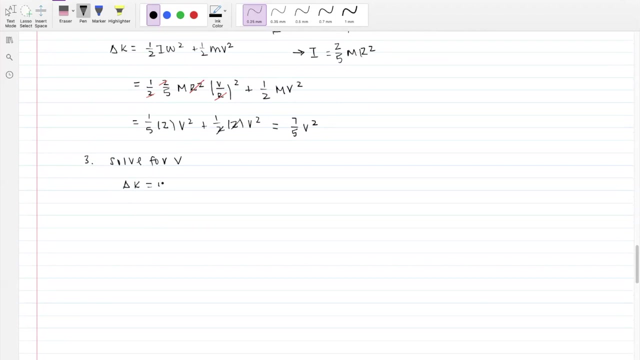 So that's going to simplify even further- to 7 fifths V squared. Lastly, now we're going to solve for velocity. So we have: delta K is equal to 400 joules, which is now also equal to 7 fifths V squared. 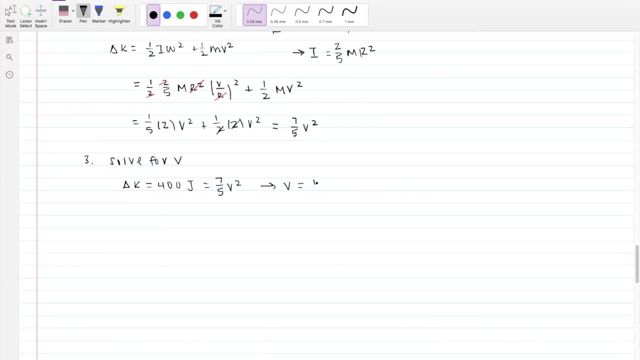 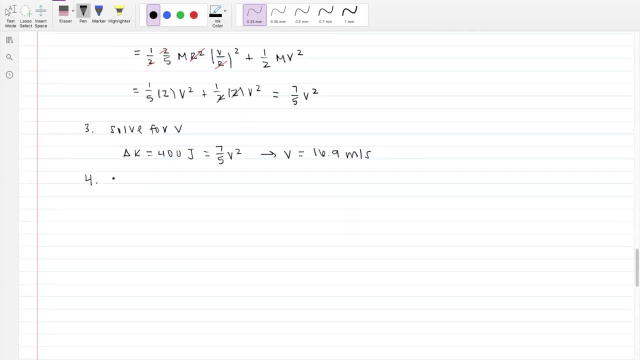 That means that our V is going to equal to 16.9 meters per second. And if you were asked what is the rotational velocity, All you have to do is use this equation. So 16.9 divided by 5 will give you 3.38 radians per second. 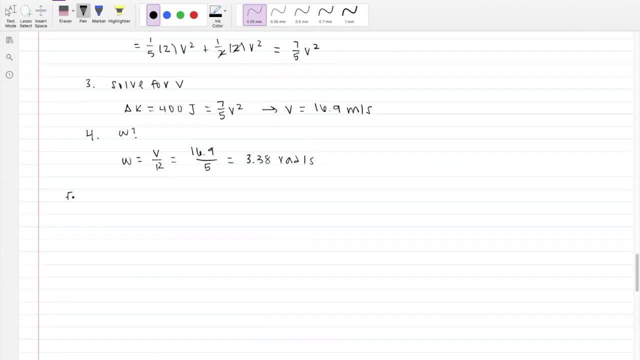 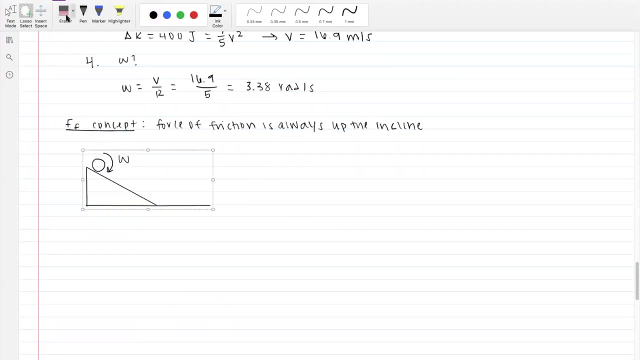 Now there are A few things I want to cover before I move on- is the force of friction concept. when it comes to rotational motion, Force of friction is always up the incline. I'm going to copy it here And actually let's move this ball down here where it's starting to roll up the hill. 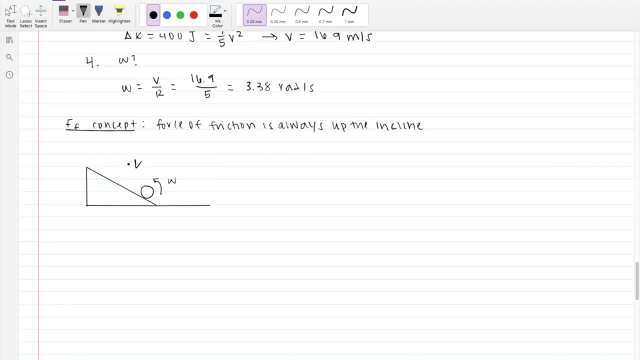 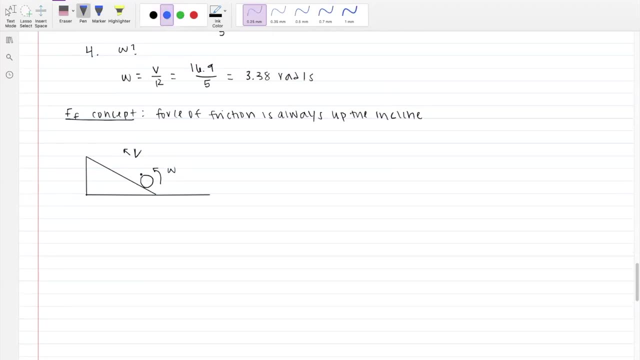 So the velocity is going up the hill When you draw your FBD. because we're considering rotation, we need to draw the forces as a given. So we're going to draw the forces as a given. So we're going to draw the forces as exact as we could. 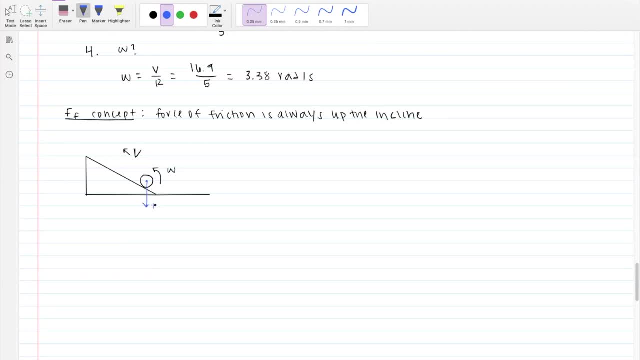 Force of gravity acts on the center of mass, So it's going to be the center of our sphere. Our normal force is being directed from the surface, Therefore it needs to be in contact and drawn all the way down to the surface. And then we also have our force of friction, which I will get to. 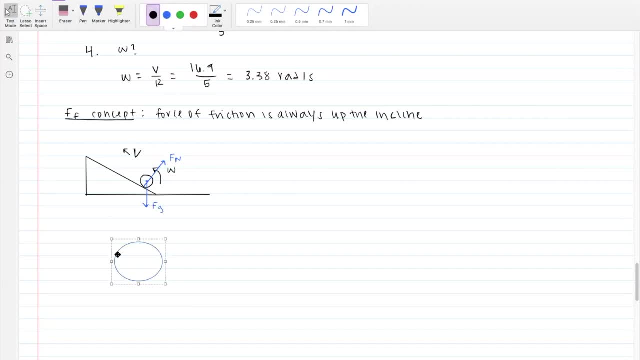 Let's draw Our sphere. Let's draw our sphere. There might be these stood peers here for a moment, as if this is actually the central surface. When you draw the force of the rock, you are not 진짜 get into it. 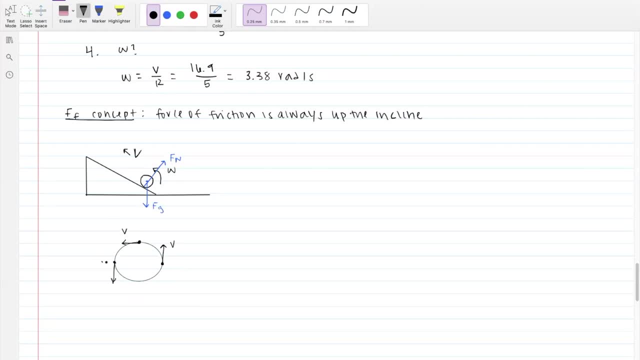 but it is strong enough for the plant to move and set up its hand over the rock. So I want you to get fully into it. When you try this out and try and acknowledge the force of friction, then you radiate the force that is being YEETed onto here. 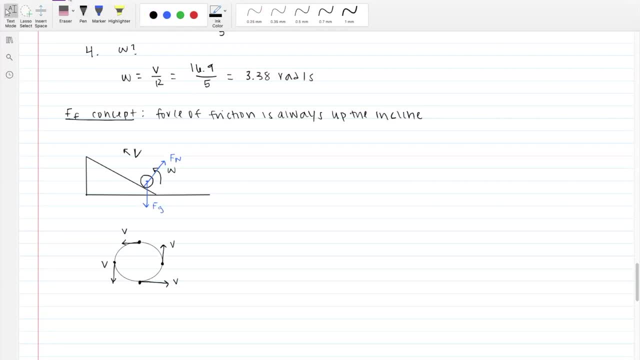 Let's recall what we honeyed out over at this point. We know that eventually, that the sphere will reach its apex and no longer have any rotation. So that means that all of these velocities at the tangents are going to be equal to zero. 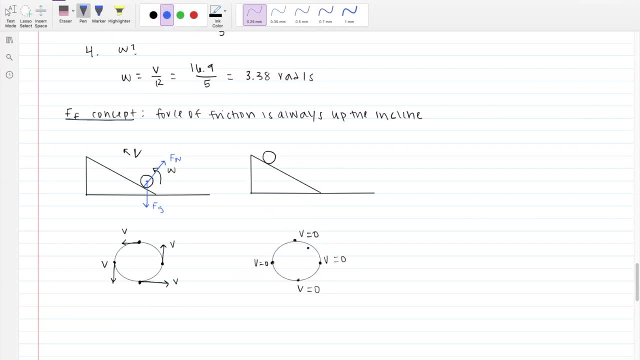 Okay, that being said, what do we know about acceleration and velocity? Very simply, remember how we said: that if our velocity is in one direction and our acceleration is in the same direction, we are speeding up, And if acceleration is in the opposite direction, that means we are slowing down. 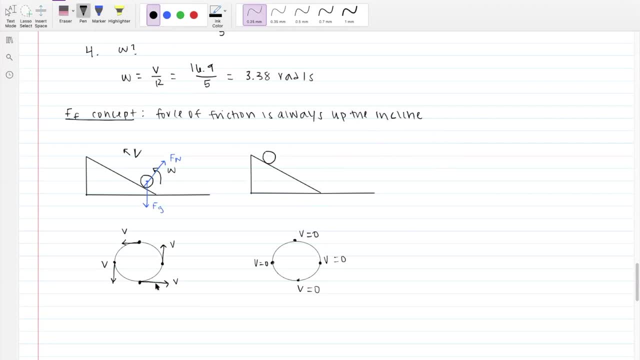 Well, that's the case that we have here. We have velocity at this tangent point which comes in contact with the surface, And if we have velocity at this tangent point, we have velocity at this tangent point which comes in contact with the surface. And if we have velocity at this tangent point, 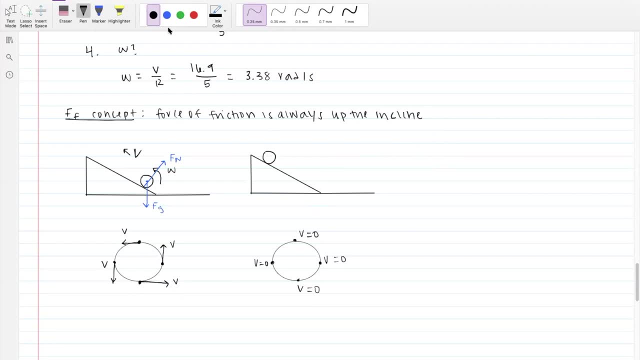 we have velocity at this tangent point. we have velocity at this tangent point is going to the direction to the right. That means for this object to slow down, force of friction needs to oppose that motion. So if we see here the velocity, the tangential, 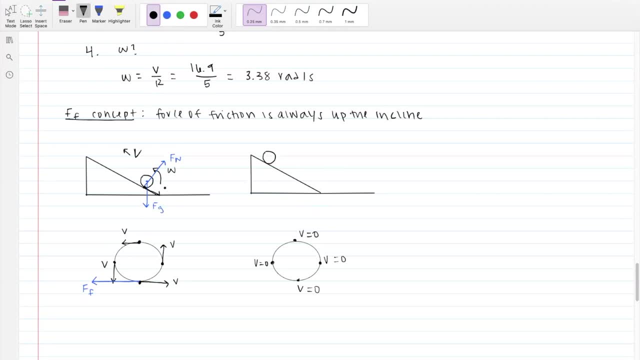 velocity which will appear here. this is the velocity of the center of mass. tangential velocity appears here. So that means our force of friction needs to be opposing that, Because this force of friction is acting in the opposite direction of your velocity. 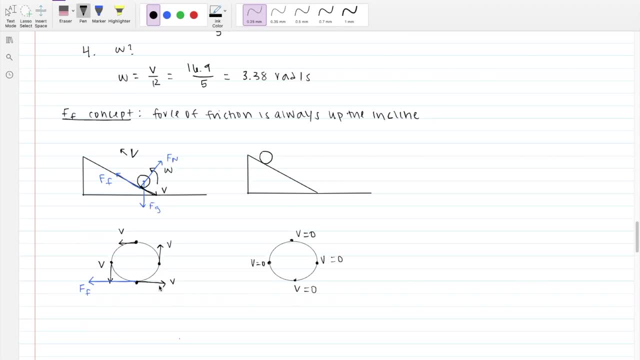 what will happen is that your velocity will then slow down and eventually reach zero, And therefore at the top of its apex we'll have an angular velocity of also equal to zero When the ball starts rolling down the incline with some sort of angular motion. 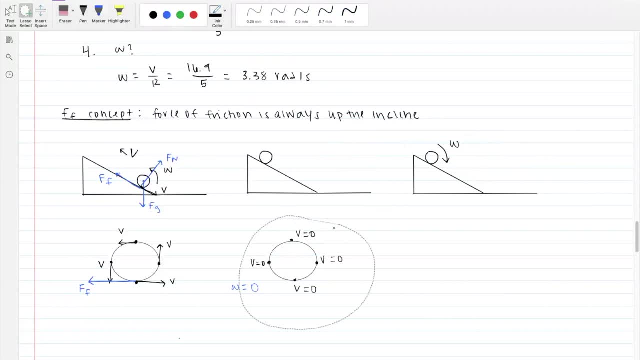 we'll see that the rotation of this sphere is going to be false. So we'll see that the ball is going to be to have is in the clockwise direction. So that means our tangential velocities will look like this And, as I said before, to go from a velocity of equal to zero to then start speeding up. 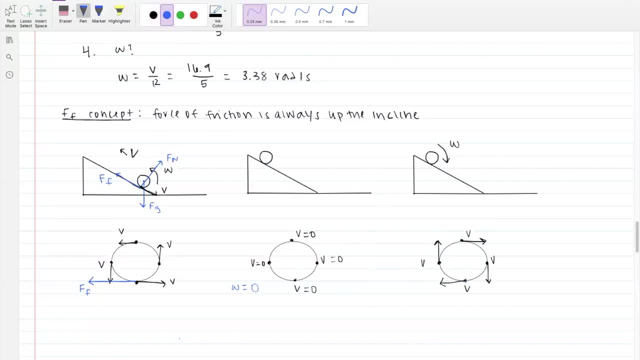 we will then need a force acting, or an acceleration acting, in the same direction as our velocity. So that means that our force of friction is going to be directed in the same direction as our tangential velocity. So, that being the case, when we draw our FBD. 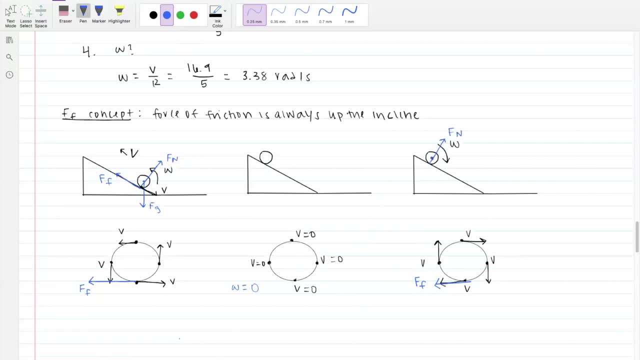 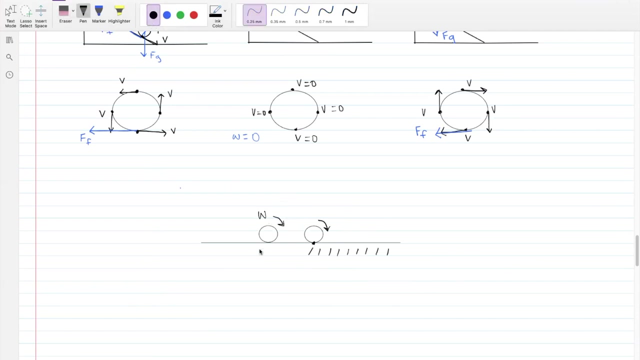 we have our normal force, we have our force of gravity and then, lastly, we have our force of friction, which is going to be still up the incline. Now let's look at the scenario where we have rolling ball that is on a smooth surface and then eventually gets onto a surface. 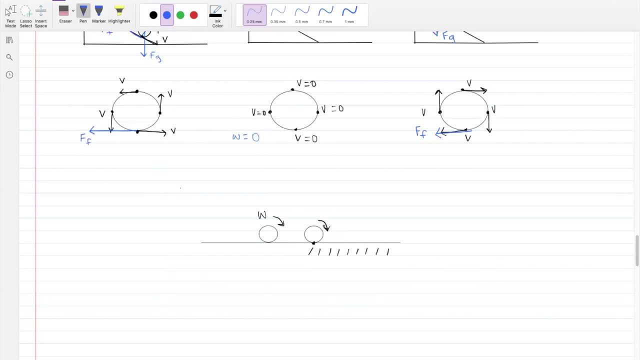 that's really rough. So let's draw our forces So we have the normal force and we also have force of gravity acting down and eventually we know that the ball will stop rolling and eventually it will stop. That means that our force of friction has to be working in the opposite direction of our tangential 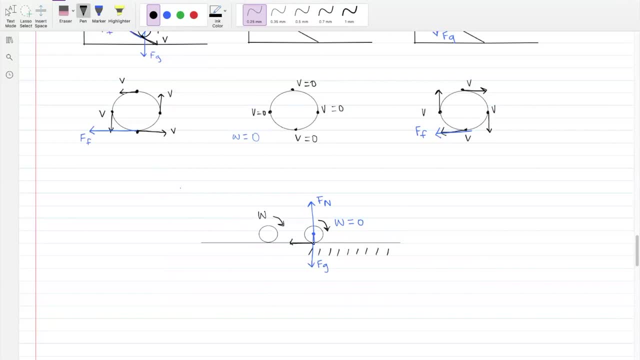 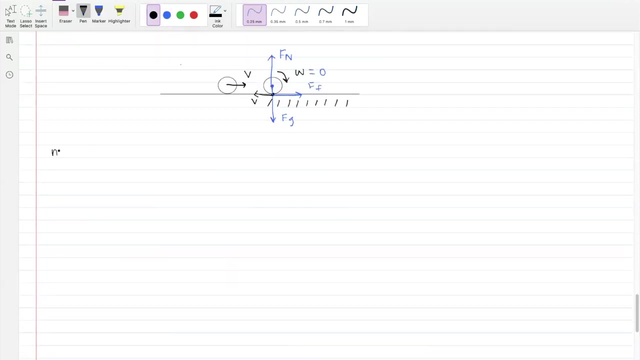 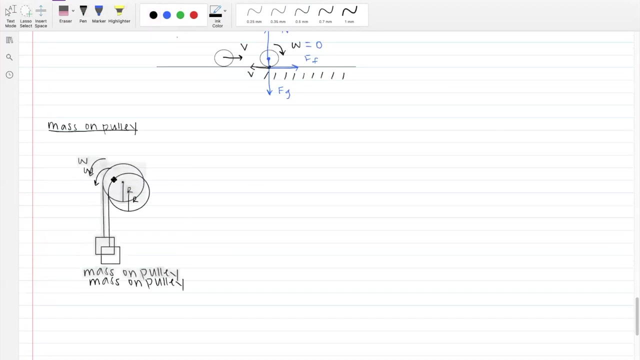 velocity. So if we have a tangential velocity here, because again the ball is rotating in a clockwise motion, that means our force of friction needs to be acting down In this direction. Now let's look at the scenario: mass on a pulley. So this is most likely the case where the 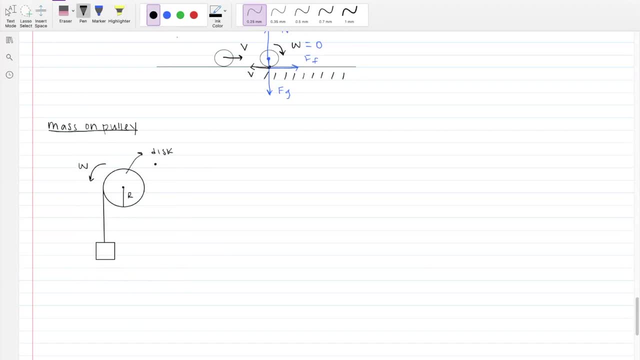 mass of the pulley is in the direction of the pool, and so this is the scheme that we're looking for. So this is a disc with some sort of mass, let's say 16 kilograms. Now, previously, in kinematics problems, we neglected the mass of the 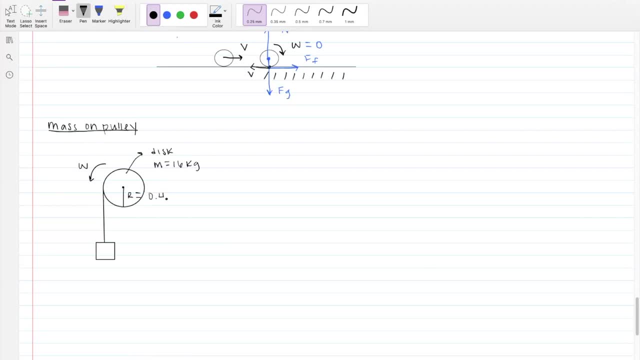 pulley. Usually in rotational problems, we don't neglect the mass, hence why it rotates. Let's say that this radius is equal to 0.4 meters acceleration of the two kilogram block. First thing you want to do is draw your free body diagram. 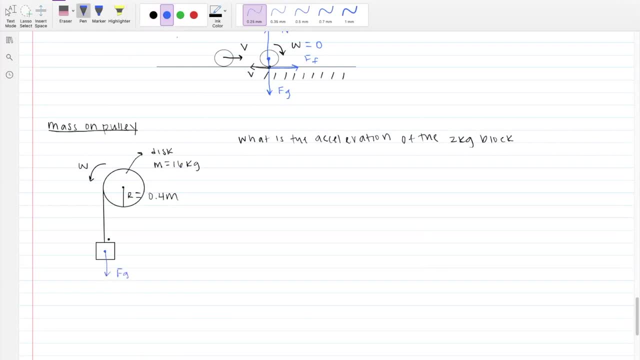 So you have force of gravity acting on this mass. You have the force of tension acting, pulling up on this mass. You have the force of tension being applied to the pulley. Now there is a force of gravity being applied on the pulley because it has mass. 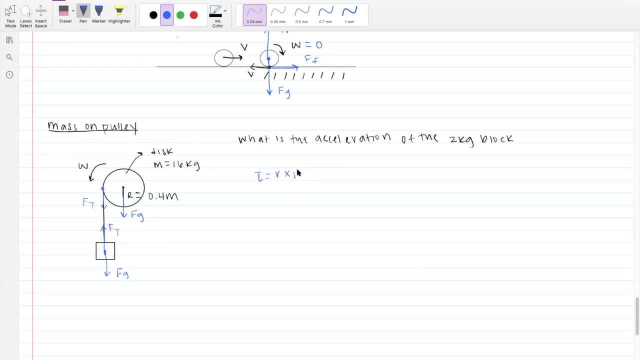 But if you remember the torque equation, torque is equal r cross product f. Rr, in this case for the force of gravity, is equal to zero. So I'm just going to go ahead and erase that vector, Because these are equal in magnitude and opposite in direction. 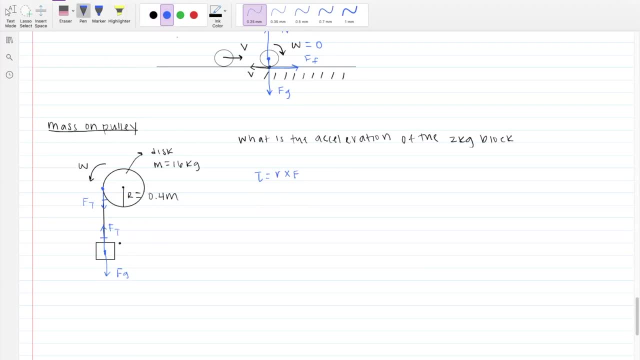 we can see that these sums, these forces, are going to cancel. So, as you see, the only force that is causing this rotation of this disc is going to be the force of gravity. So let's look. Torque is equal to r, cross product f. 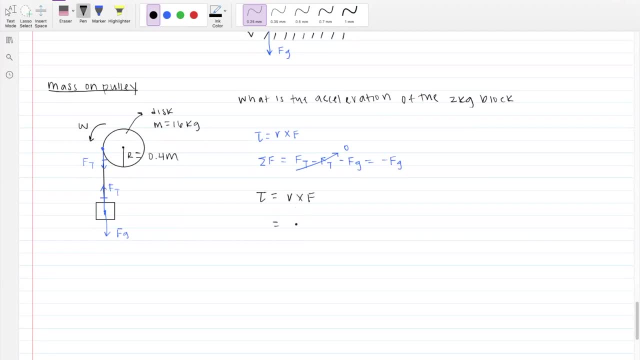 We have a radius of r, which is 0.4, and the force that's being applied, f of g, So that's going to be 10 times the mass of the block. So this is going to be times 2.. So this is going to give us 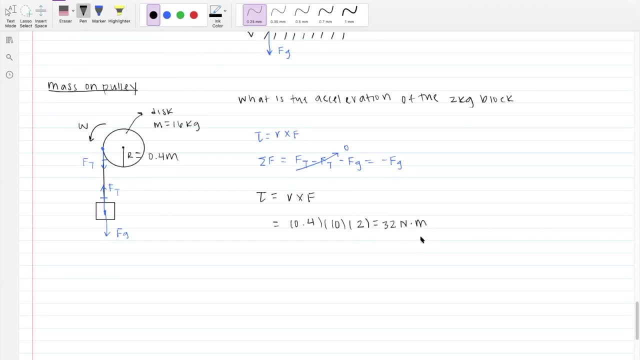 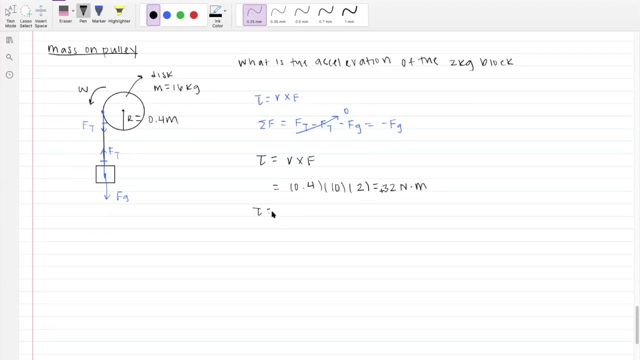 32 newton meters. Again, I did assign a direction to this force, But what we really consider is the fact that this is rotating counterclockwise. So we're going to consider this torque positive. Now, torque is also equal to moment of inertia. 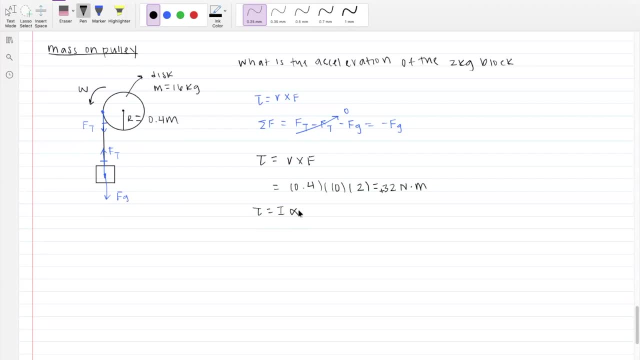 times times alpha or angular acceleration, and the moment of inertia for a disc is equal to one half m r squared. So that's equal to one half times 16 times 0.4 squared, which is equal to 1.2 kilogram meters squared. 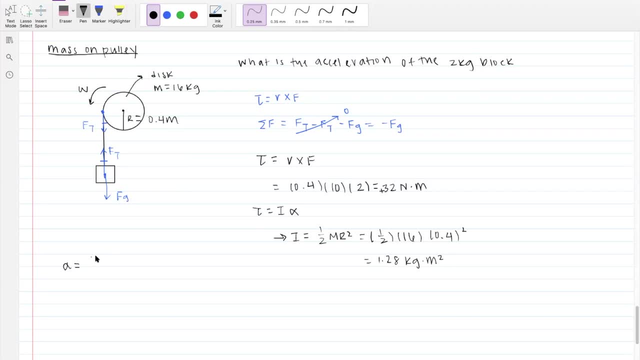 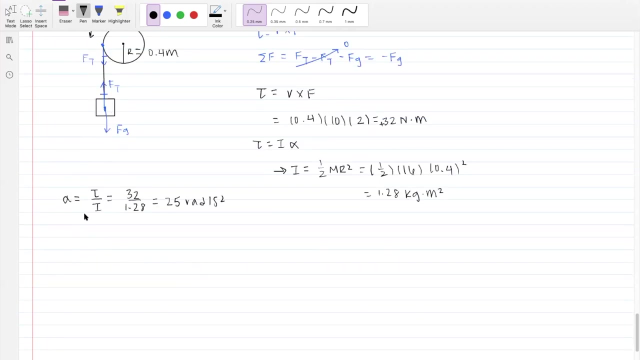 So therefore, our acceleration- we rewrite this as torque over moment of inertia- is equal to 32 newton meters. over this, 1.28 kilogram meters squared, which is going to equal to 25 radians per second squared. And to go from angular acceleration to acceleration, we 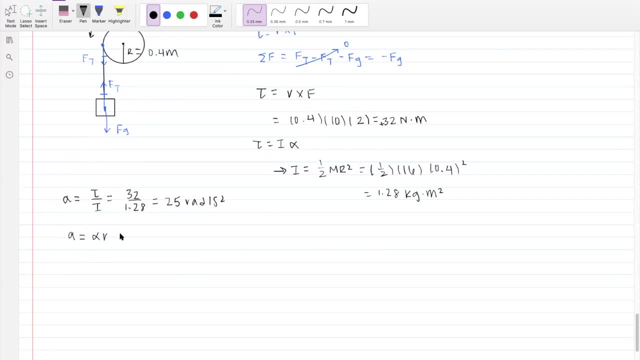 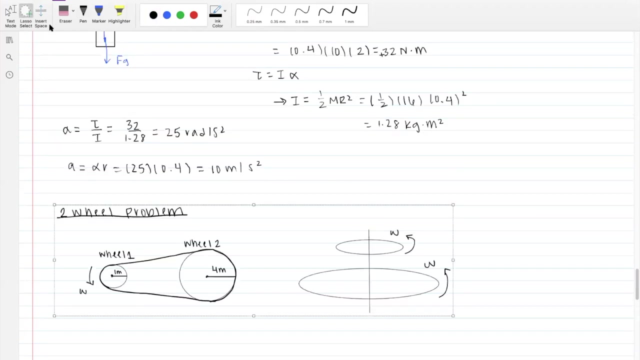 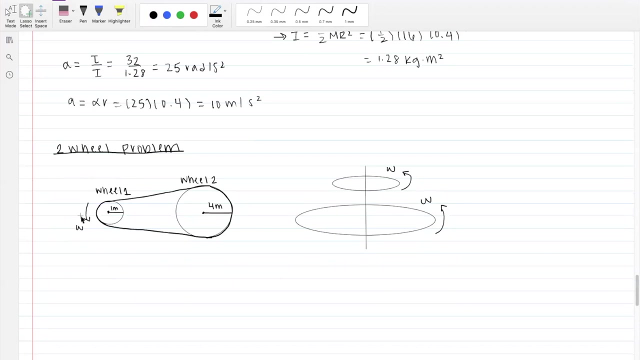 have, acceleration is equal to alpha r, so that's going to be 25 times our radius, which is 0.4.. That's going to give us 10 meters per second squared. And lastly, we're going to look at the two-wheel problem Now. I've seen cases where we 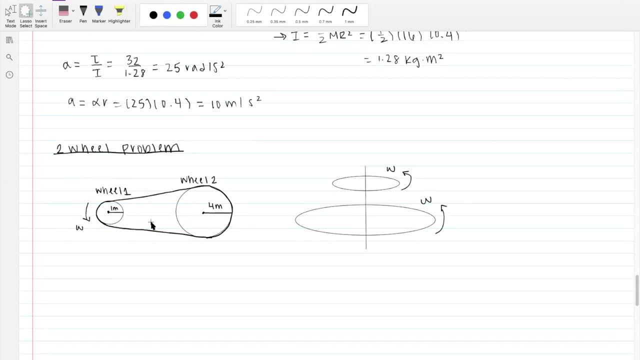 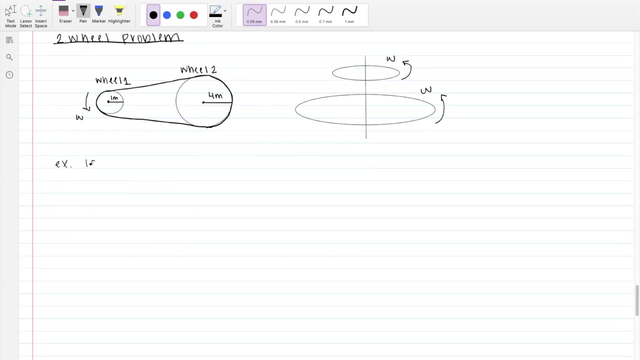 have a string that is attached to both of these wheels. I've also seen wheels that are rotating about some sort of connected axis. Either way to solve these problems is the exact same. So let's do an example with problem one. If w2, the angular velocity of wheel 2, is equal to six radians per second, 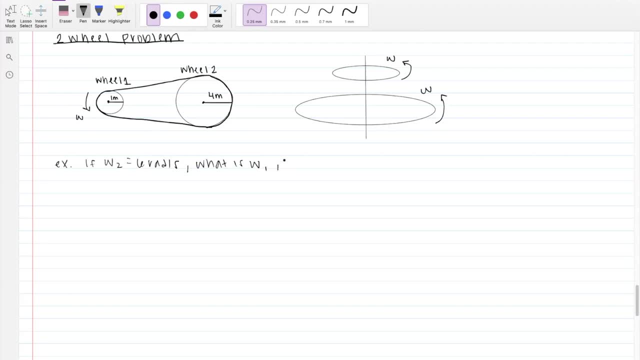 what is the angular velocity of wheel 2 per second and the angular velocity of wheel 1?? Is that the exact same? Let's ask a simple question of wheel one. given that the mass of wheel one is two kilograms, the mass of wheel two is equal to three kilograms. 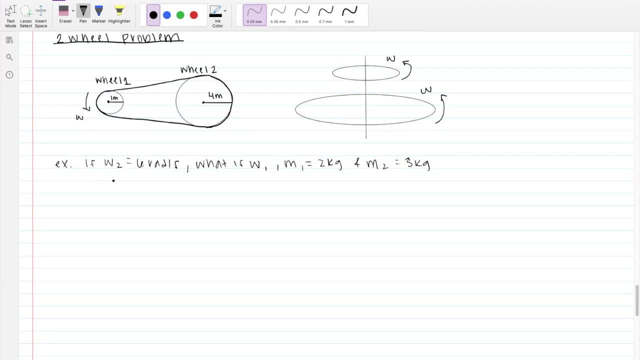 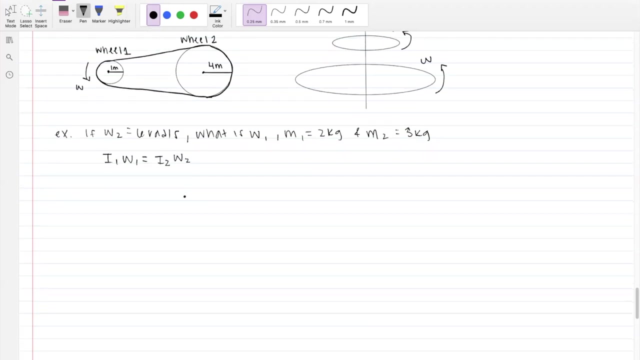 Whenever you see a two-wheel problem, the first thing I would think of is: okay, I probably want to use my conservation of angular momentum equation. And we have that. these are discs, So the moment of inertia for a disc is equal to one-half m r-squared. 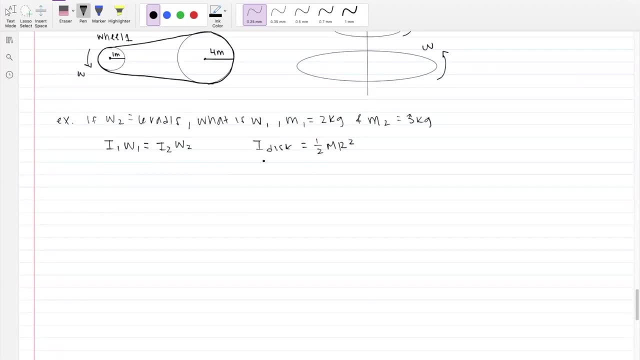 So I1 is equal to one-half times two times one squared, which is equal to two kilogram meter squared. I want inertia for wheel two. So I1 is equal to one-half m r-squared. I2 is equal to one-half three times four squared, which is equal to 24 kilogram meters squared. 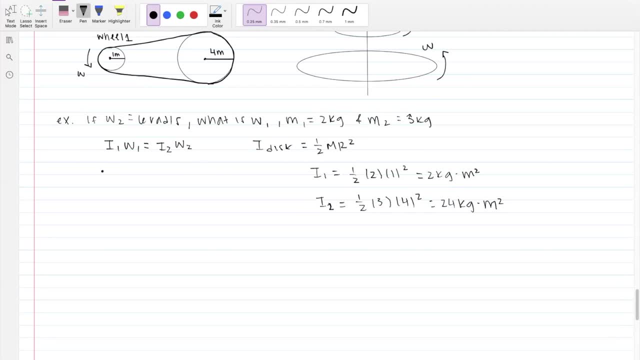 So let's plug in these values. So we have moment inertia for wheel one, So that's two. We don't know its angular velocity yet. We also have 24 for the moment of inertia for wheel two And we have angular velocity, which is six. So the angular velocity for wheel one.